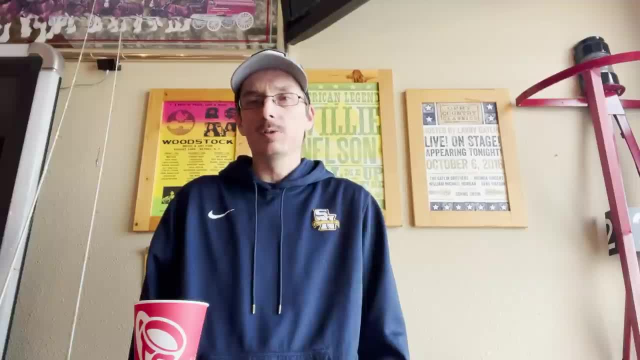 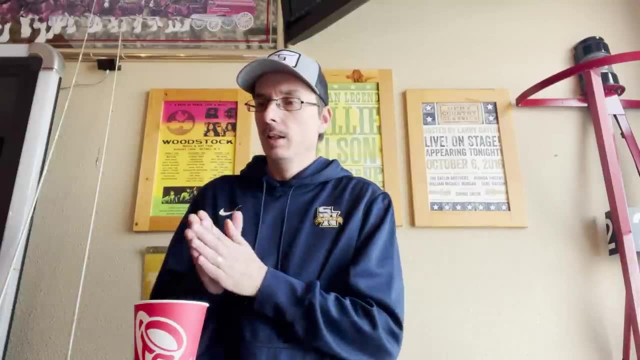 in the water and in some locations I know a lot of times even in Milwaukee, Wisconsin, you know this can be a little bit different, even time frame. sometimes they'll fish all the way up to the first of the year and then they get their boat in the water again in February at some point. but for most places this is. 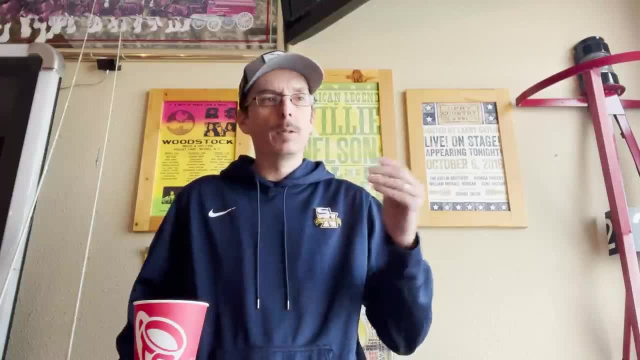 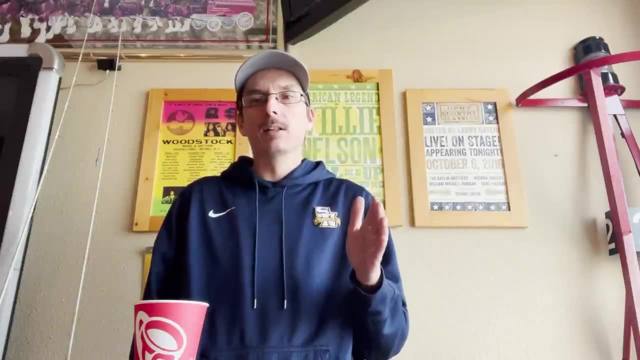 going to be true that sometime in mid-march or so you're going to be able to launch your boat and go out and chase after spring browns, and that spring brown trout bite is going to last until the alewife come in to spawn- and when is? that well, that could depend on the year. some years it's mid-april, some years it's end of April, some years it's beginning of May. but basically what happens in Lake Michigan is the alewife will come in to the river systems or the shoreline area to spawn, and when they do that, they basically flood the shoreline. 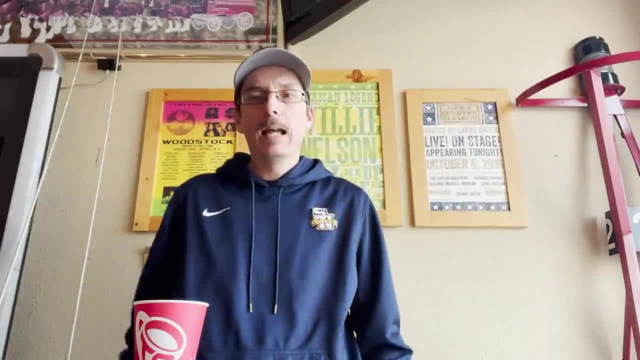 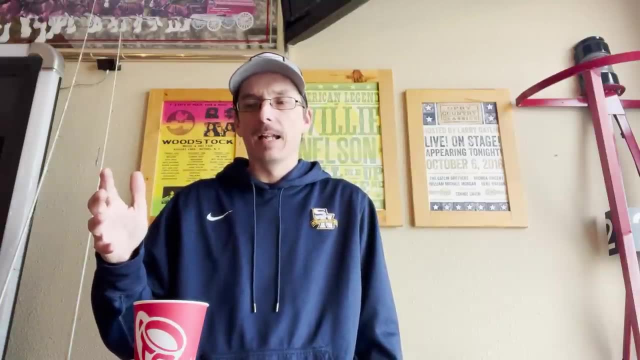 to the point where your graph will go out. you'll see nothing but bait and you obviously just can't compete with artificial equipment, artificial tackle, with the, with that kind of bait fish very well. so what will happen is, you know, we'll have really good brown. trout fishing, generally speaking, from anywhere from about four weeks to six weeks- it'll kind of last- and then that'll be, like I said, anywhere from generally about mid-march all the way through till mid to end of April. it's pretty regular from year in and year out. the locations that we generally target: 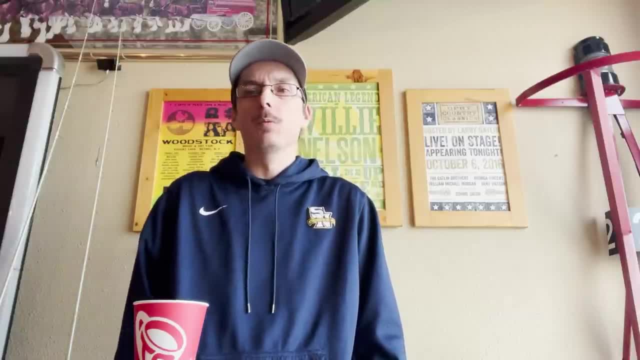 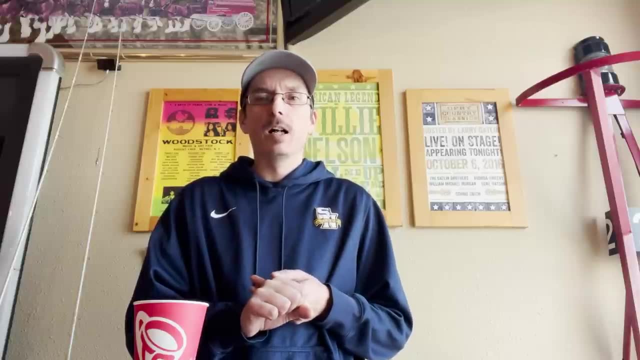 depending on what ports you're fishing out of, but this kind of goes, for most ports are going to be one of three locations. basically, one is a harbor or river mouth area. if you have a river that dumps into the lake, that may be warmer than the. 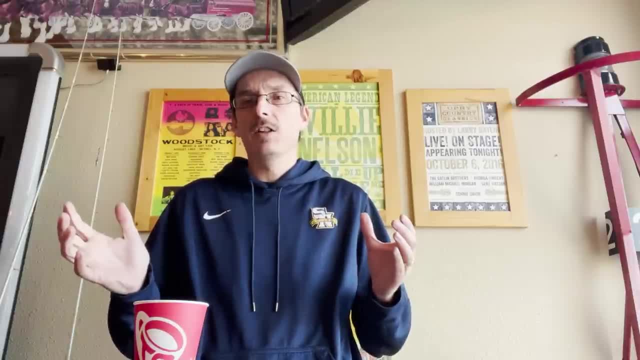 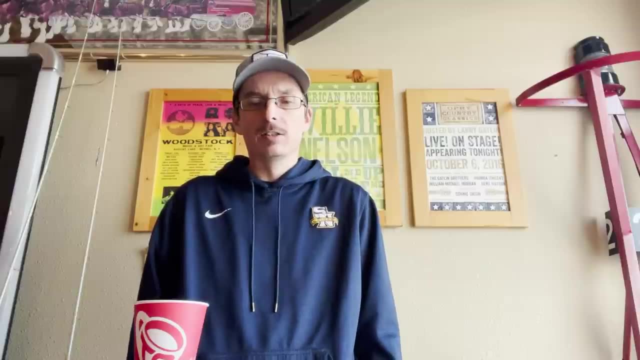 lake water a lot of times in the spring, especially all kinds of fish, just not brown trout, coho salmon, king salmon, you know all kinds of fish will congregate towards that warmer water. that's a great location to start looking. I've caught hundreds and hundreds of brown trout in and around the Sheboygan Harbor area. 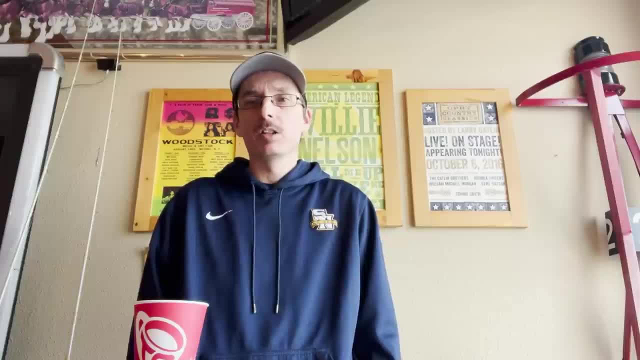 it's a great location to take a look if you have a warm water discharge of any sort from a power plant or a water plant or whatever where you may have a warm water discharge that pumps into the lake, where you'll create a warm water area, one of the most premier brown trout. 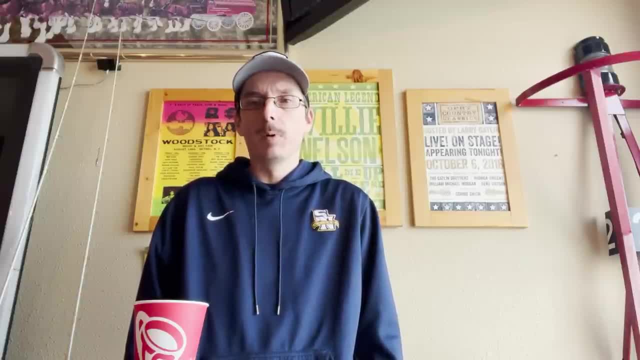 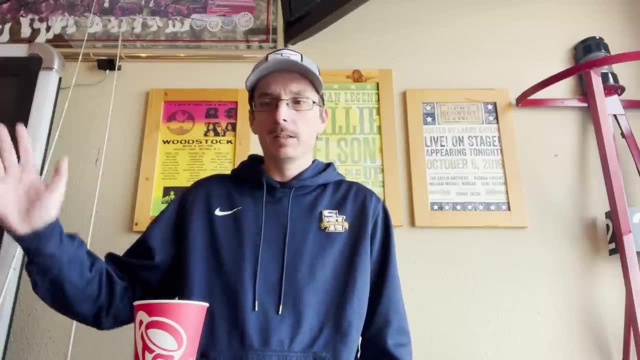 locations in the country is by the Oak Creek power plant, where they have some warm water that that pumps in, and what's interesting about that is that's a. that's a location, whether it be the Oak Creek one or other ones, where you know it's not as easy as they're always saying. it's a good place to start and 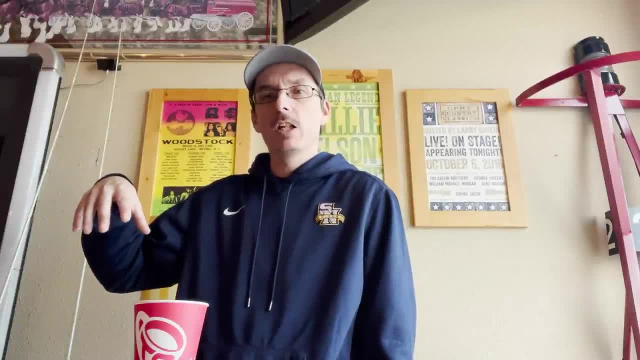 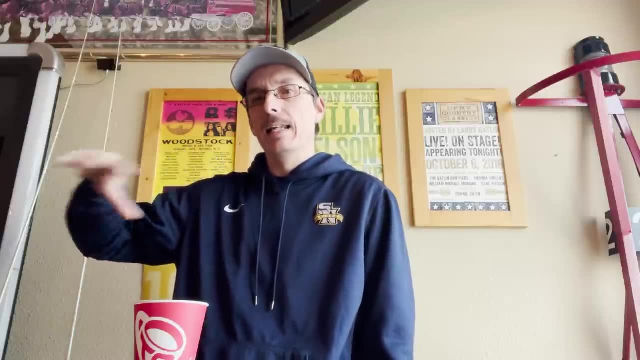 always sitting right in the hot water. sometimes that's too much of a change for their body, so sometimes they'll be around the edges, where the water might be a few degrees warmer than the rest of the water, but not in the middle of it. so you got to take a look. you'll be looking at these. 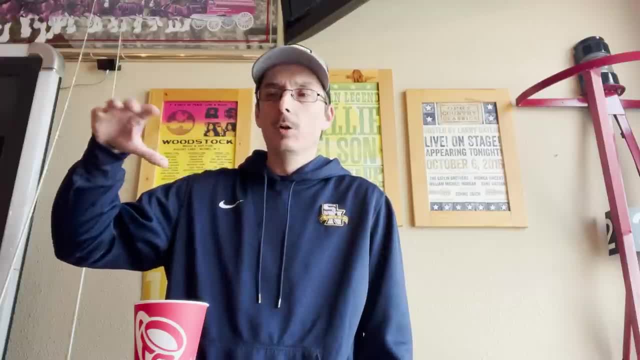 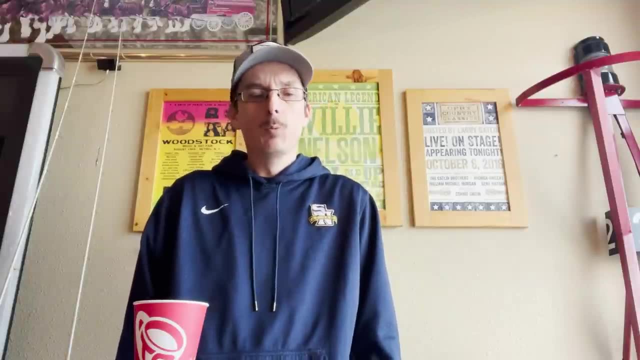 harbor mouth areas, maybe even inside the harbor area. you'll be looking at these warm water discharges and then really in the last 15 years, as the forage has changed tremendously, what we've been finding here out of cheboygan and i know in a lot of ports, is areas where you have a lot of 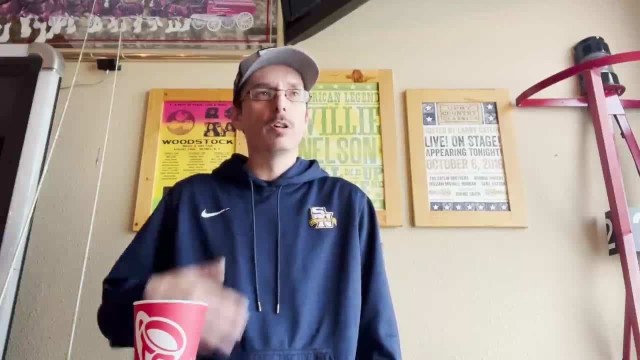 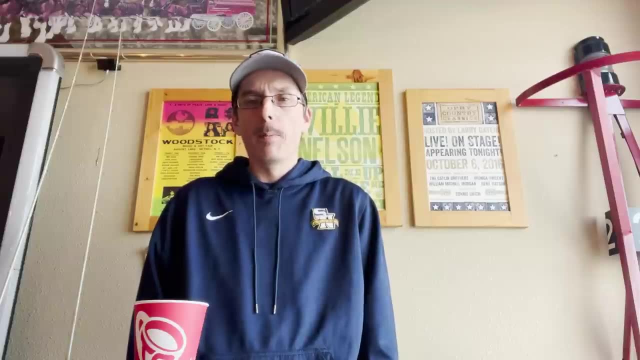 rock and big boulder tend to be really good. so here at cheboygan we go north of the harbor and fish up by the whistling straits, golf course a lot, and that seems to be, you know, probably our premier location, for here in cheboygan it would be our oak creek power plant to milwaukee, you know. 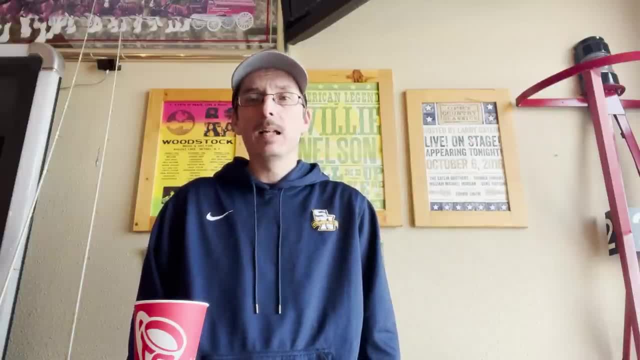 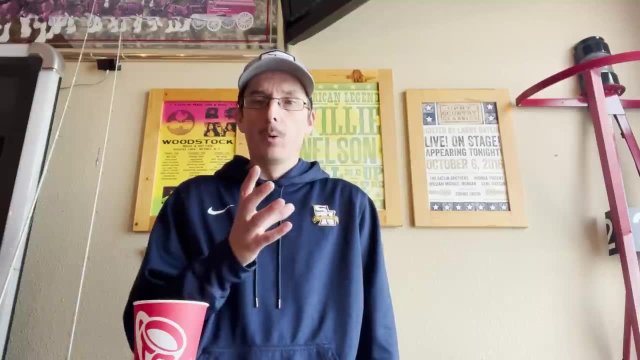 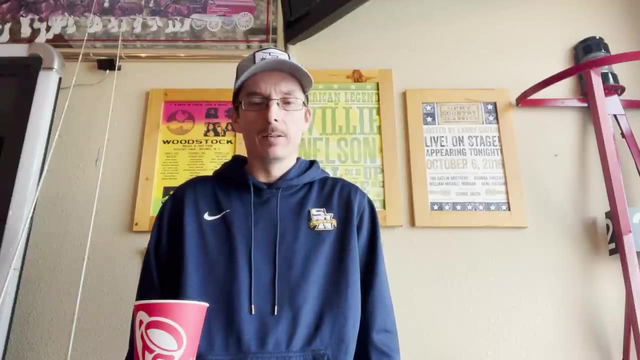 that would be our, our premier location, and the reason being is that the main forage now for brown trout is the goby, the round goby. so it also the round goby is dictating our location. it's also dictating our tackle. um, we're making a lot of different decisions now than we used to, based on on the round goby. so 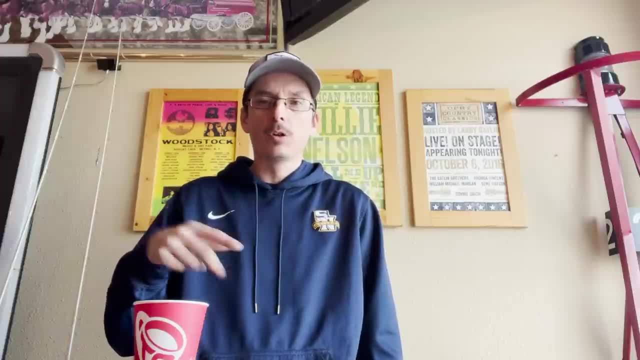 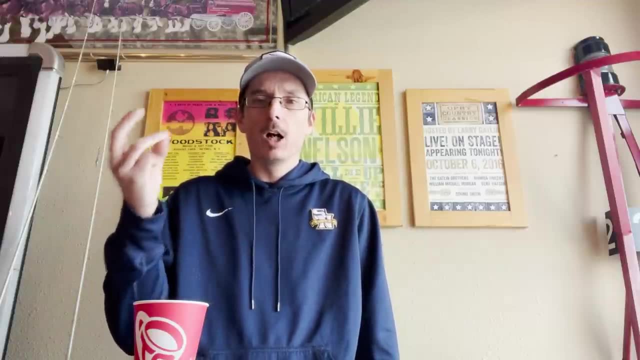 three locations you're going to look for for this spring, when you're going to fish brown trout, which is coming up here and already what is probably less than 60 days. um, those three locations again are going to be a harbor mouth, a river mouth area, a warm water discharge, if you. 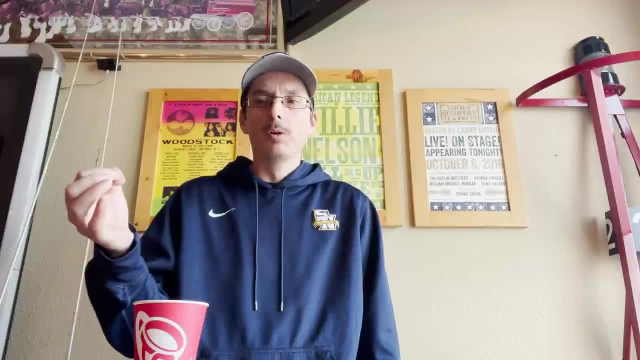 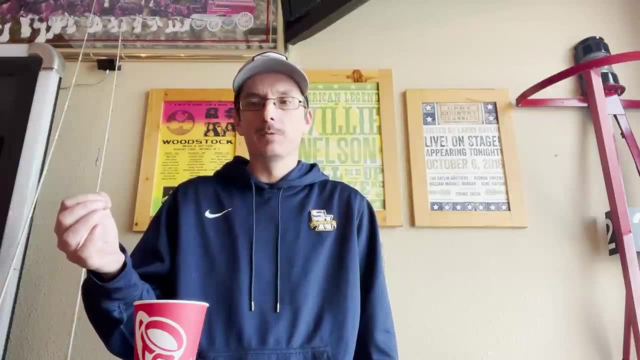 find one or areas where there's lots and lots of big boulders that'll hold a good, healthy population of gobies, which will all, which will absolutely hold a good, healthy population of spring brown trout. so that is the location. now let's talk about equipment, one of the nice parts. 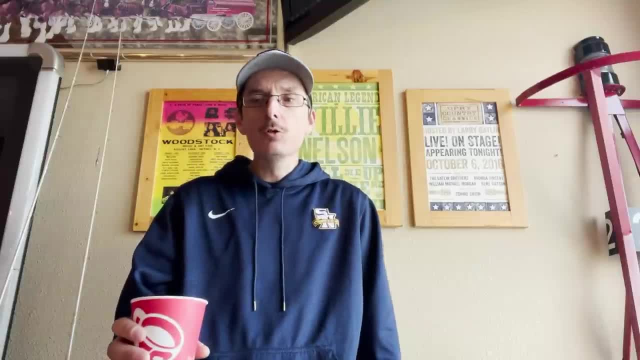 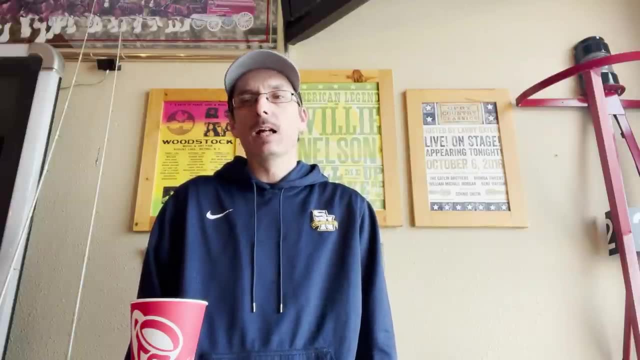 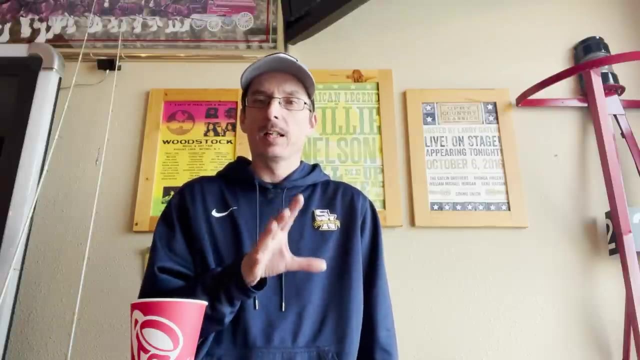 about brown trout fishing is you don't need high-end equipment or fancy equipment and you definitely don't need a big boat. it's the uh one of two times a year that i see a lot of 16 to 18 foot boats that i don't see on lake michigan a lot- and i'm talking those particular boats you can. 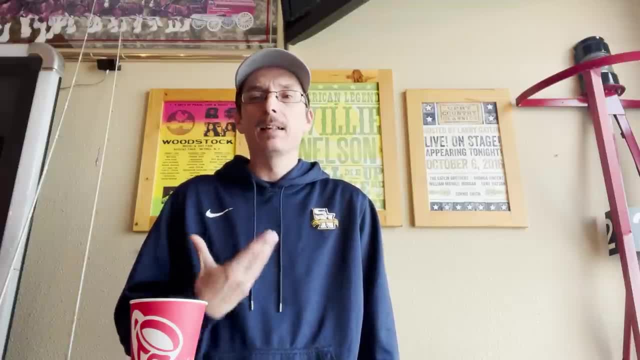 absolutely use a 16 to 18 foot and i'm not going to talk about is that you know, like the sweet foot boat on Lake Michigan, but I'm saying I see a lot of guys with 16, 18 foot boats that I only 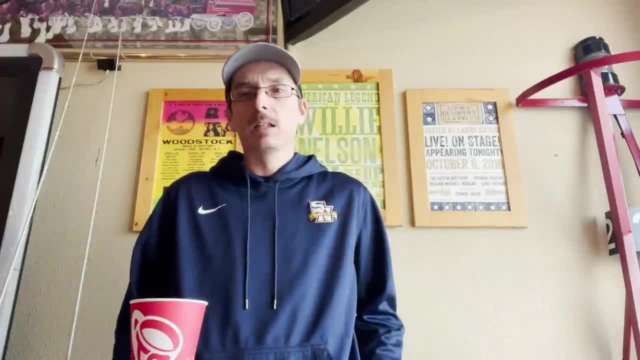 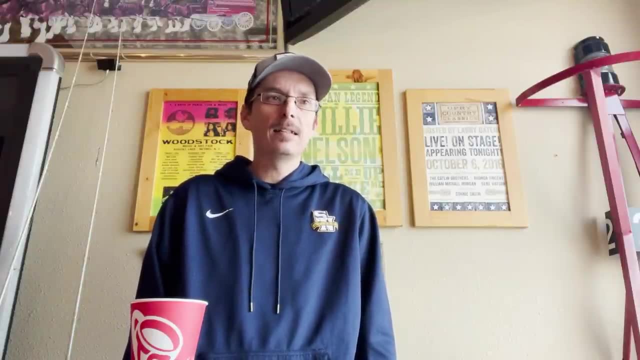 see in the spring and I only see in the fall, and the reason being is because we're fishing shallow water. Most of the fishing is done here in Sheboygan in probably 8 to 15 feet of water. In Milwaukee it might be a touch deeper than that. maybe it's 10 to 20 feet of water. 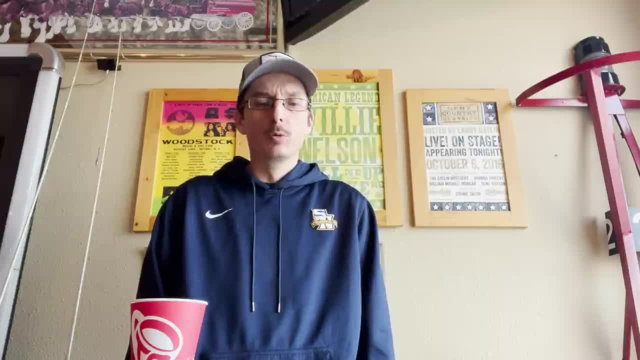 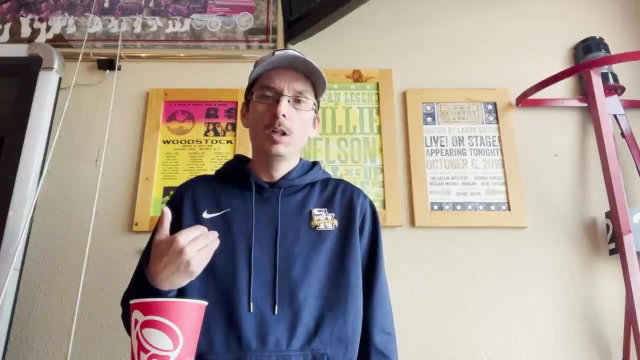 but the point being is that you're fishing almost exclusively in 20 foot or less when you're tacking spring brown trout and because of that you're fishing very close to the shore. so people feel very comfortable in multiple sizes of boats. So if you own a walleye boat, that you go walleye. 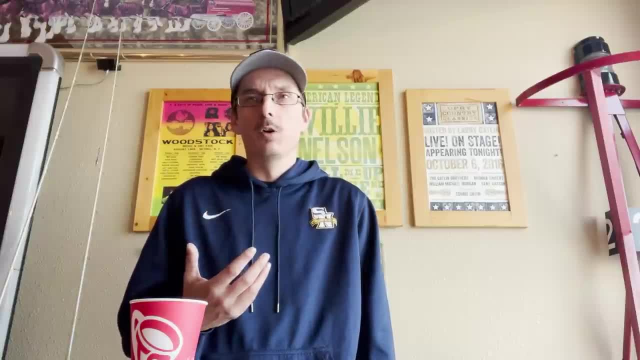 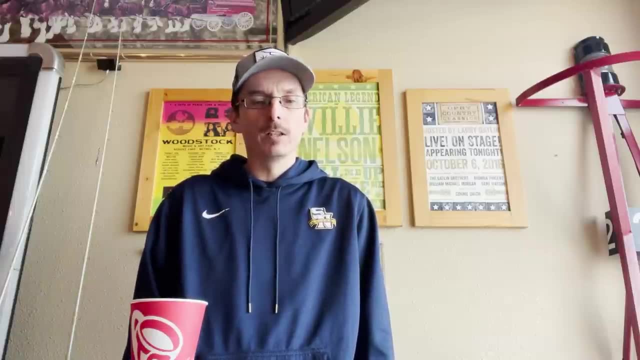 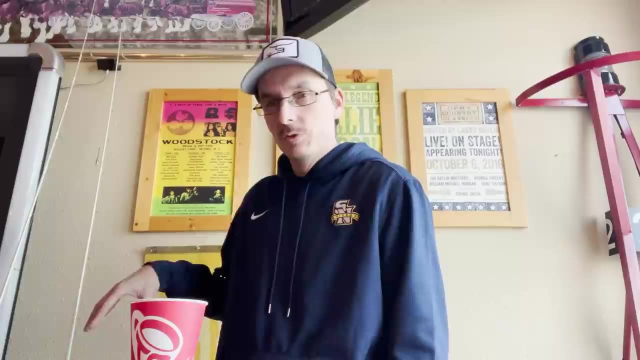 fishing with a 16 to 18 or 16 to 20 footer and you own some walleye trolling rods and reels, you can definitely, with a few lures, go out there and have some fun catching brown trout. So I'm going to show you some of the basically walleye rods that my dad uses on his boat when he goes. 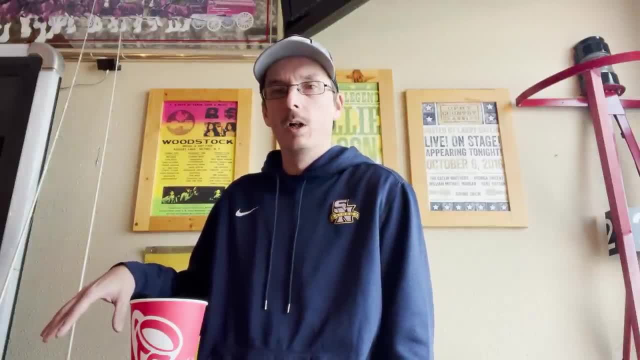 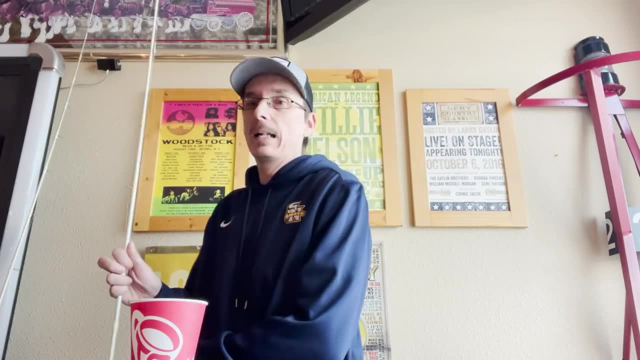 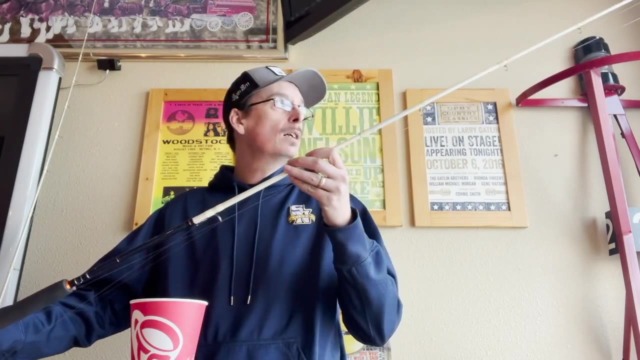 spring brown trout fishing and how we've converted those to make those work for brown trout fishing, which is exactly the way I would do it if I was going to rig up brand new equipment. So this particular rod here is a Okuma white diamond. it's probably a downrigger rod. it's a eight foot medium action. 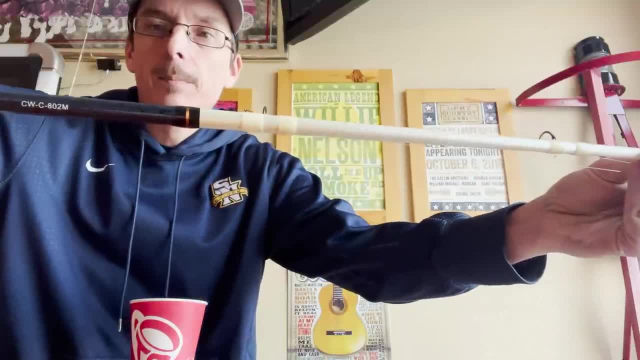 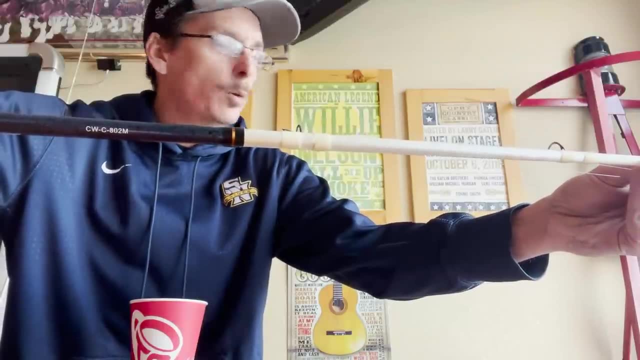 Okuma. see if I can maybe get that on there. yep, so that's a. I'm sorry. yeah it's a. it's an Okuma cold water eight foot medium rod. it's a downrigger rod. we use it as a planer board rod. 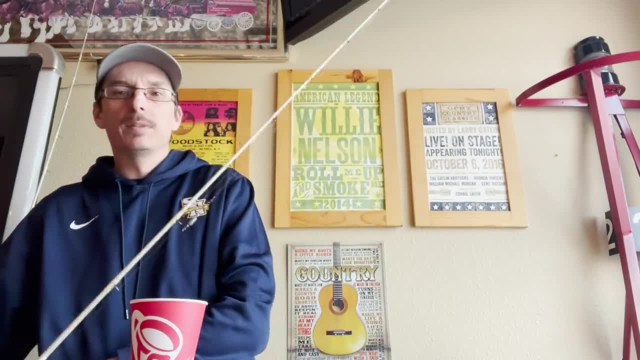 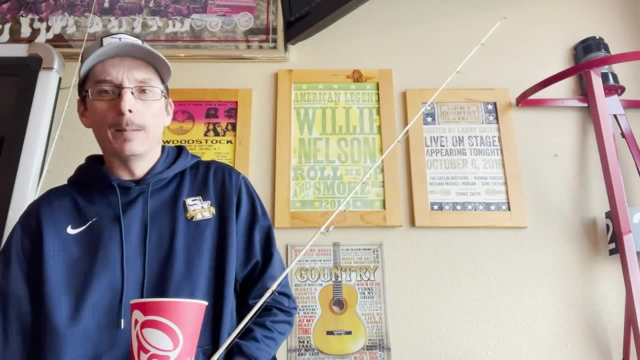 it's got a very, very soft tip, which I think is important. this is a very, very soft rod. I think that's very important when it comes to brown trout fishing and the equipment that we're using. we're using 20 pound braid as our main line, because that's the same line that my dad uses. 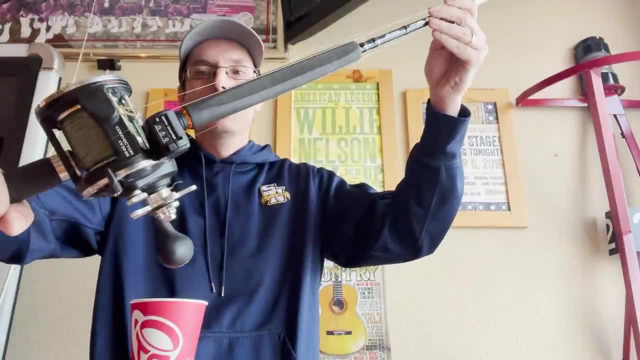 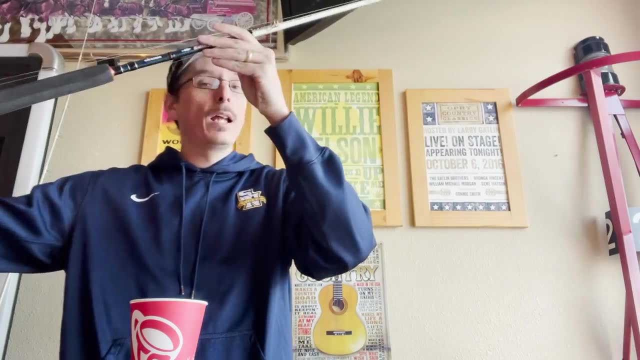 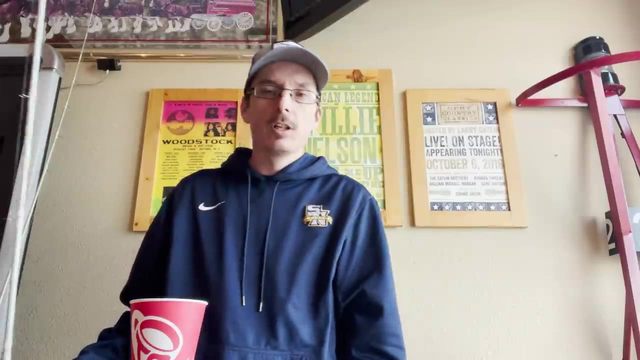 for walleye fishing. I'm just trying not to catch anything here, so so there you can see he's got 20 pound braid as his main line on an Okuma convector reel and for walleye fishing and spring browns, and that he prefers the high speed that's a convector 30 ds, because you're not, he's not hauling anything. 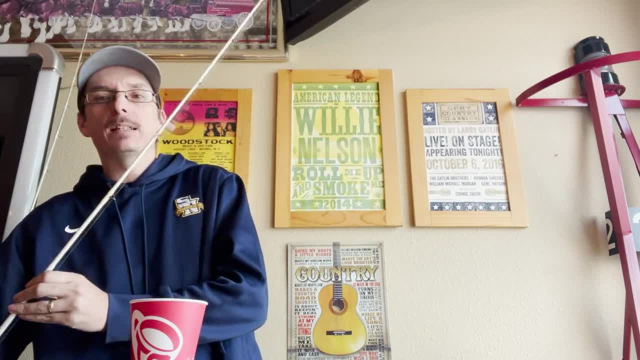 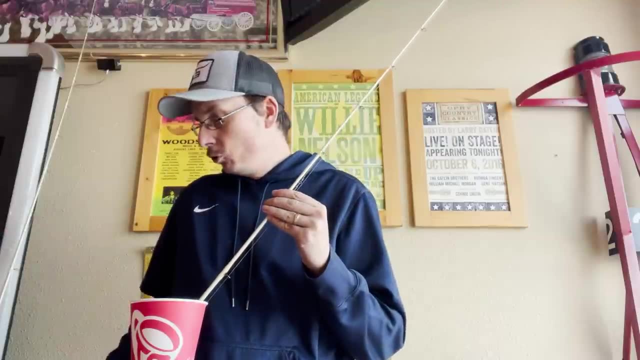 you know heavy. he's not toying coppers with these setups or magnum dipsies or anything like that, but he's going to have six of these planer boards rigged up, and then he's also going to have two mini slide divers rigged up, so he's going to be able to run a total of up to eight rods. 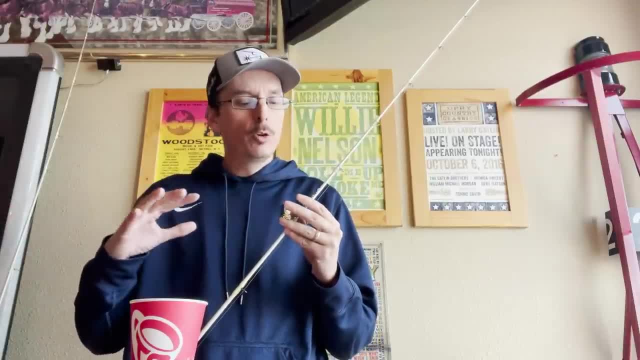 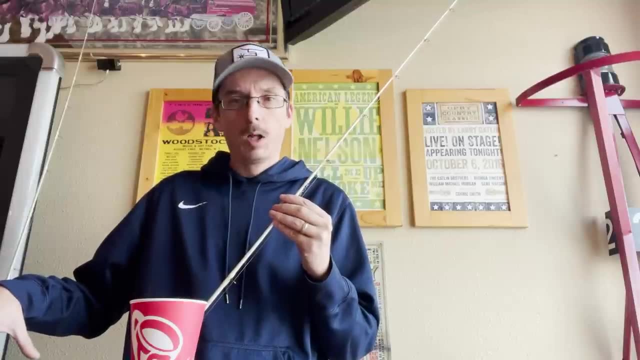 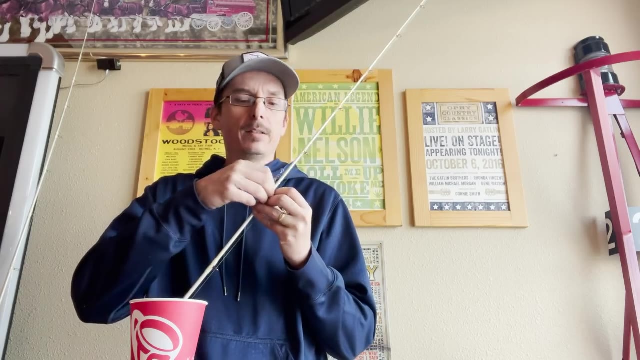 if he takes three people on the boat. so let me show you kind of the planer board set up to start out, with the 8 foot rods, cold water rods with a convector, 30 ds reel and 20 pound braid. it's got 20 pound braid all the way to the swivel. we got a standard, you know, salmon candy- 55 pound ball. 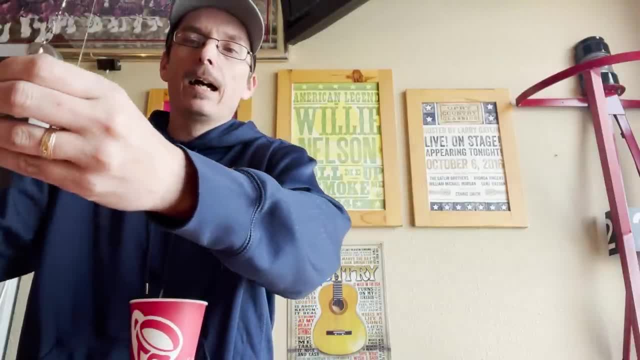 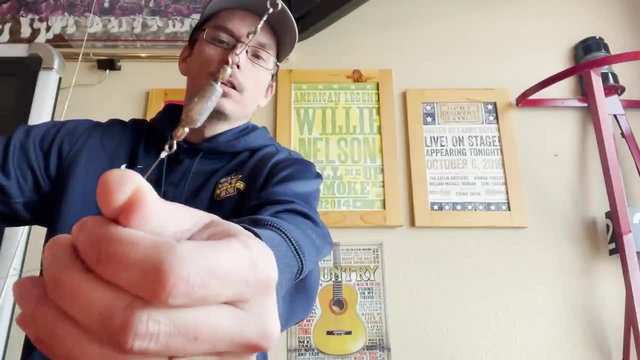 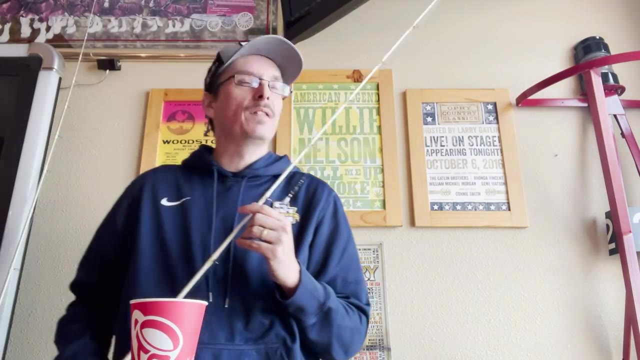 bearing swivel on there, but from the swivel we have a quarter ounce inline sinker. some people call them a torpedo sinker. it's an inline sinker, that's all it is, and quarter ounce is really smallest ones you can possibly find. quarter ounce is the smallest i've ever ran into, if i could find. 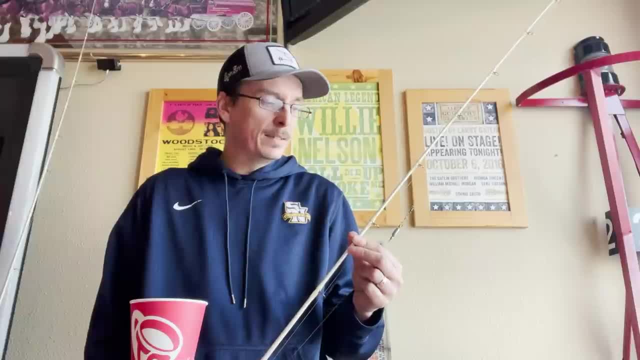 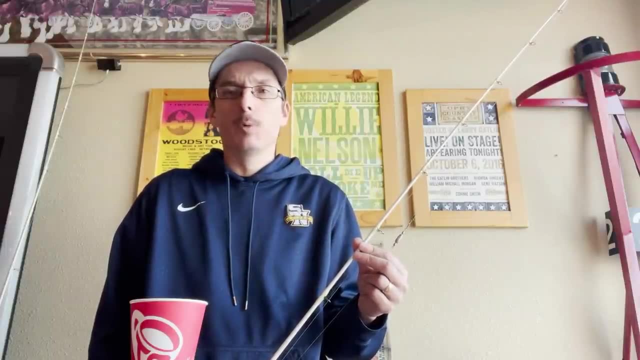 an eighth ounce, i would um the smallest ones you basically can find, because, as i mentioned before, we're fishing in very, very shallow water. uh, here in sheboygan, 8 to 15 foot, i would say is the most common, so you're not able to let very much line out at all before you're into the bottom. so, having 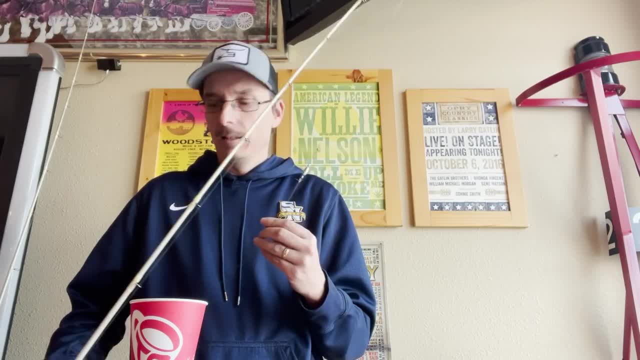 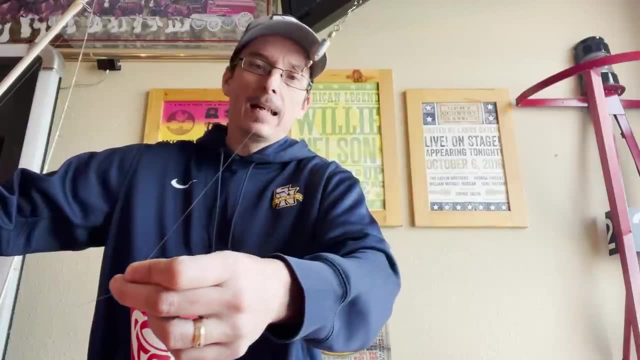 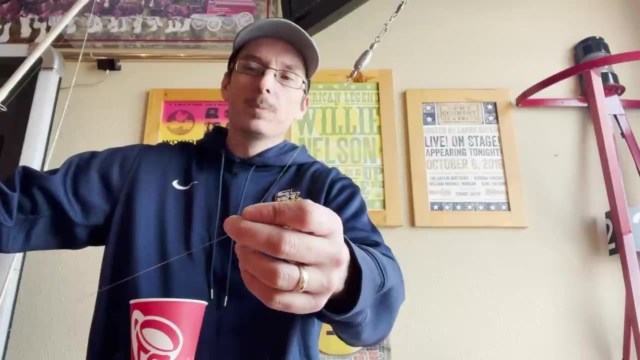 the least amount of weight, the better. and then after that on this setup he's got a monoliter monofilament line, probably 15 pound test. if i had to guess, this is one of the very, very few times you're going to hear me say something less than 20 pound test for spring browns, because the average 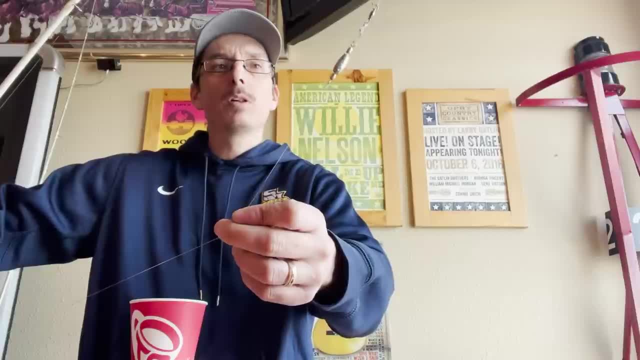 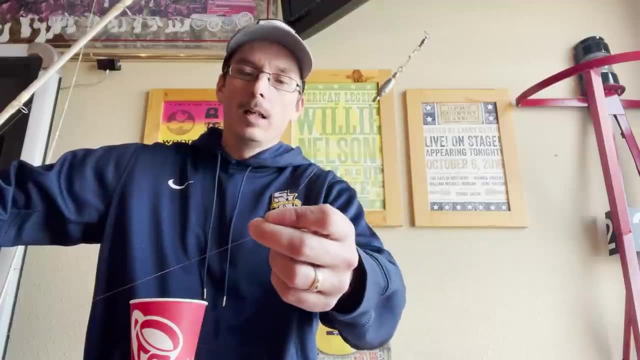 size of them are probably four or five pounds. you might catch a 20 pounder but in general you're going to deal with a lot of four, five, three, six, eight, right in that range. pounds. 15 pound model helps run these smaller to smaller tackle very well and he usually likes a rod length, so this: 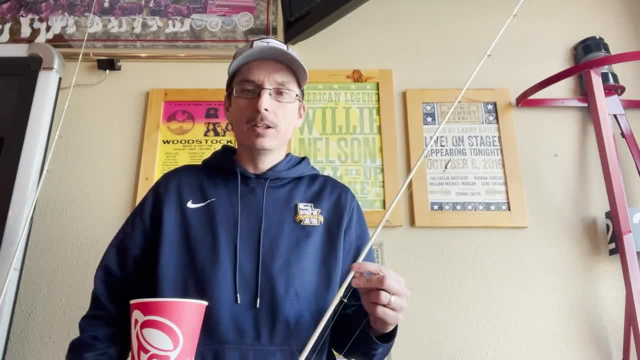 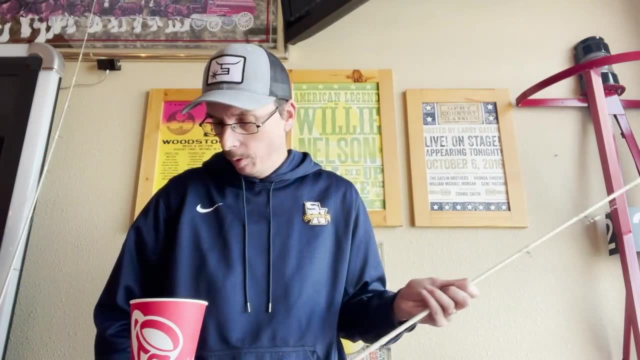 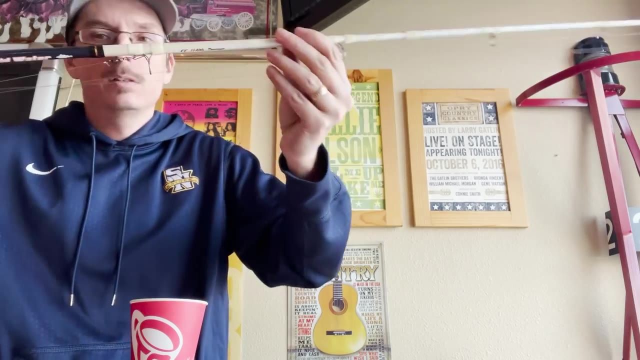 is an eight foot rod length and he usually likes a rod length and he usually likes a rod length. he's probably got an eight foot leader from his weight to another 55 pound salmon candy ball bearing swivel in which he has, i believe, attached right here to the rod tip. so there's his swivel, that's what he's. 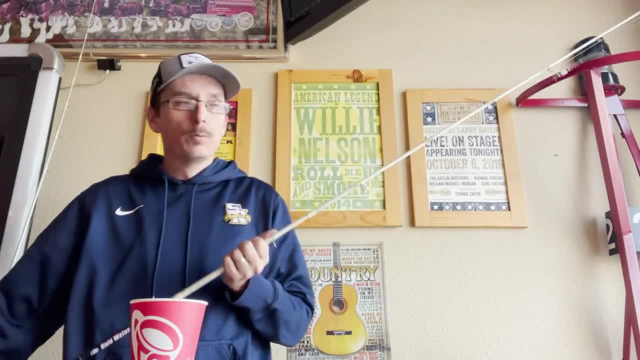 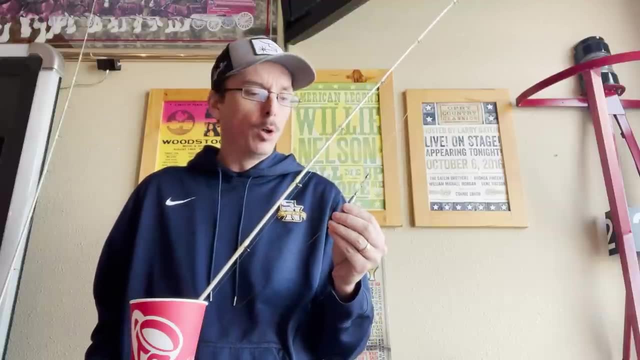 going to attach to his spoon. now, right away, i'm going to tell you you're only going to use this weight if you're going to fish a spoon. if you're going to fish a bay rat crankbait or a rod tip, you're going to use this weight if you're going to fish a bay rat crankbait. 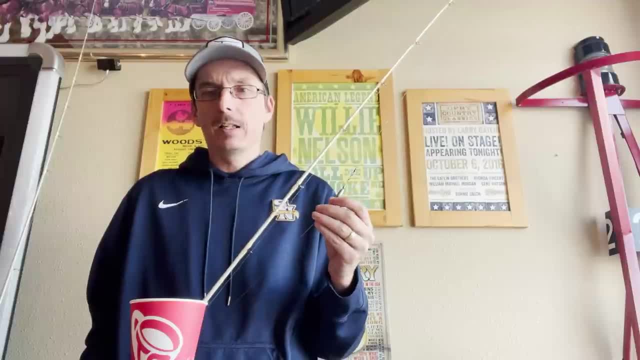 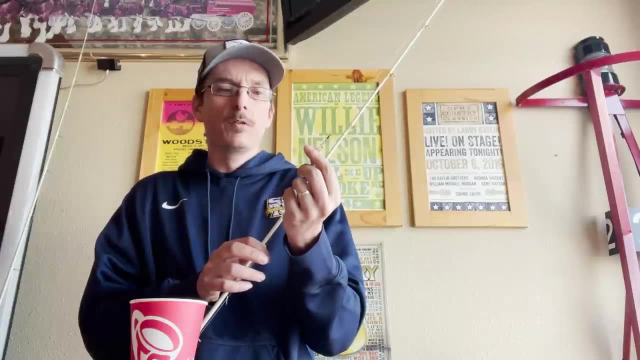 or a rapala or a husky jerk or a thunder stick or anything like that- any shallow diving crankbait- then you don't need a weight, and that's why he really likes this setup where he puts a swivel attached to the weight. you could just tie your line to it. but if he quickly wants to change over, 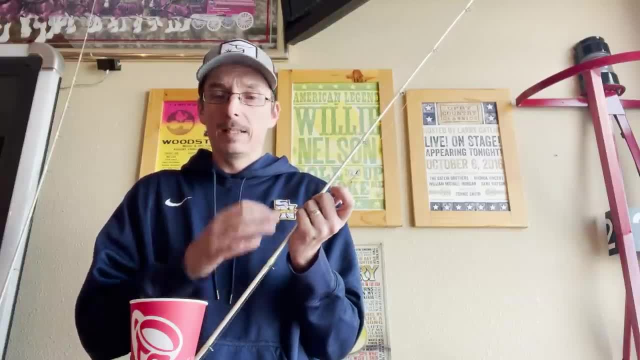 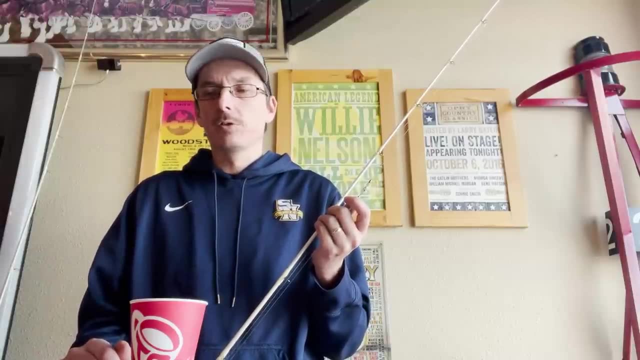 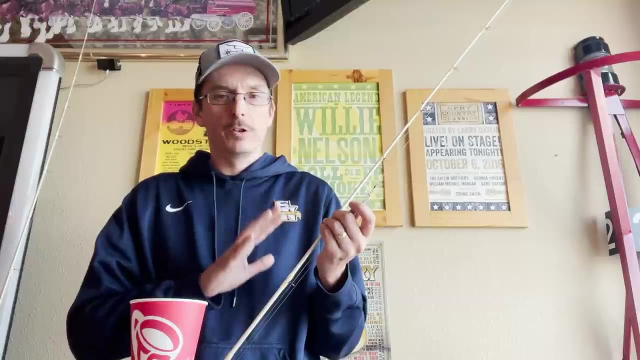 to a crankbait. he can do that. what he, what my dad and myself have found in the past 10 years is we're fishing almost exclusively spoons. we very rarely fish crankbaits anymore. we'll give them a try, but but very rarely do we fish them very much anymore. so we are primarily fishing these inline sinker setups. 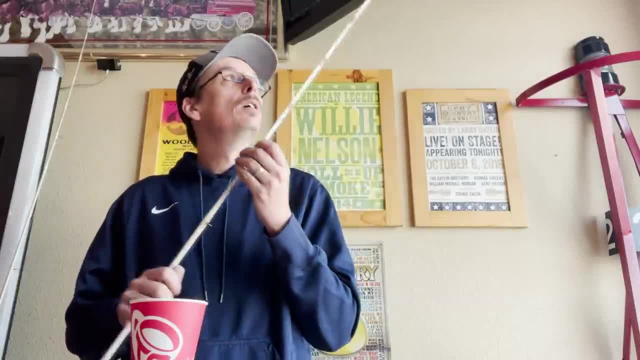 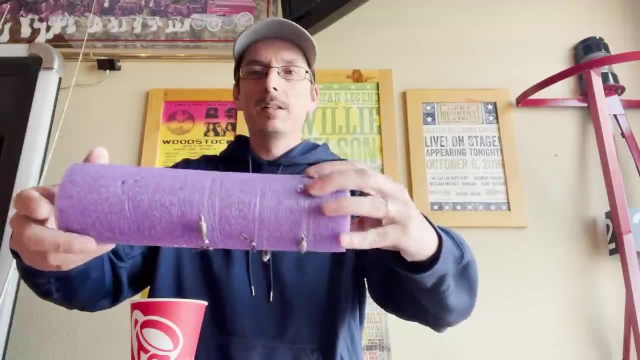 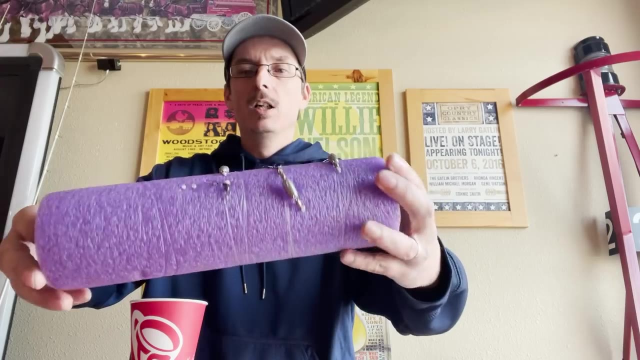 on our planer boards and we'll likely fish as many as six at a time. he does rig up these ahead of time so he's ready to rock and roll and he just puts them on one of these you know floating deals these kids floaties and wraps them around. stick some nails in there, as you can see, so that 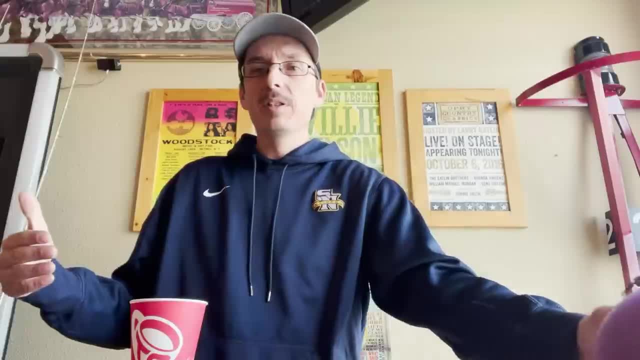 he can just quickly attach this setup. the other reason he does that is when we go walleye fishing or he goes walleye fishing. we're going to have to do a lot of work on him, so we're going to have to, so that he's got the guy on his rod and he can just put his wodge in, or i go with them, or whatever. 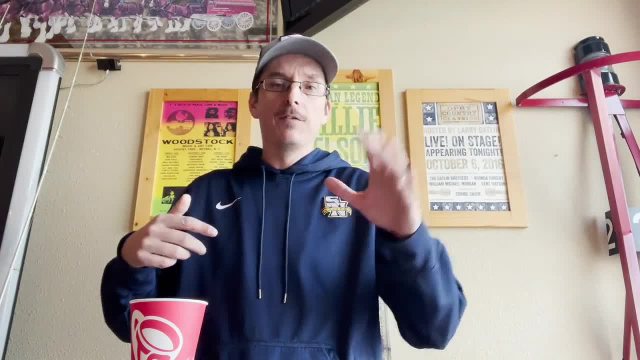 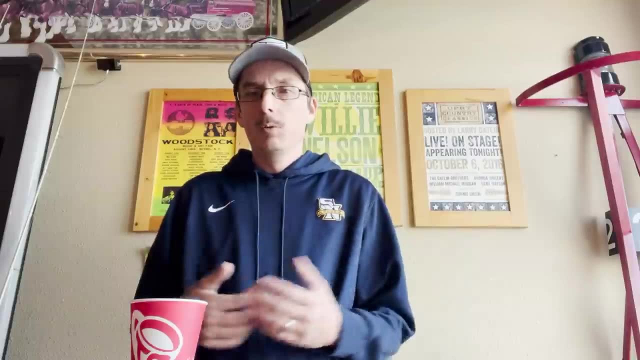 he can quickly take these inline sinkers back off, wrap them up, and now he's just got a swivel on his, on his rod, and so he's ready to put his flicker shad or flicker minnow or walleye nation's you. 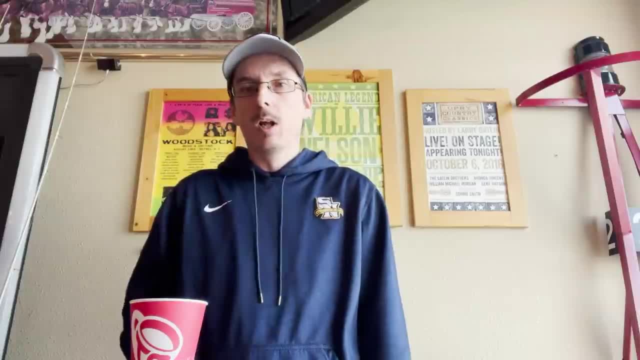 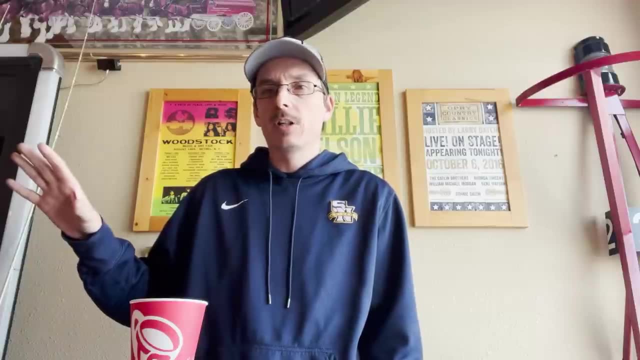 know shaky shad or whatever crankbait he's going to use that day when he goes walleye fishing or crawler harness setup or whatever he's ready to go. so again we got six planer board setups would be. our average setup takes three people. we could run up to nine rods. we'll probably run eight. 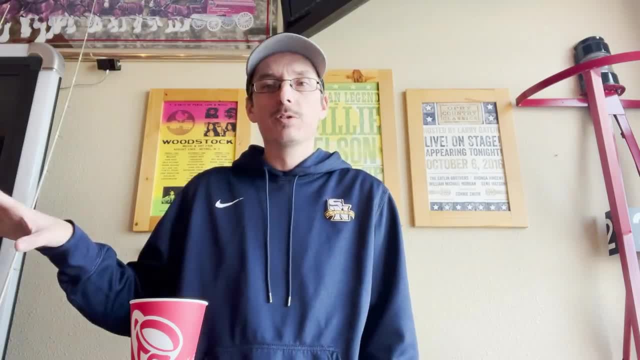 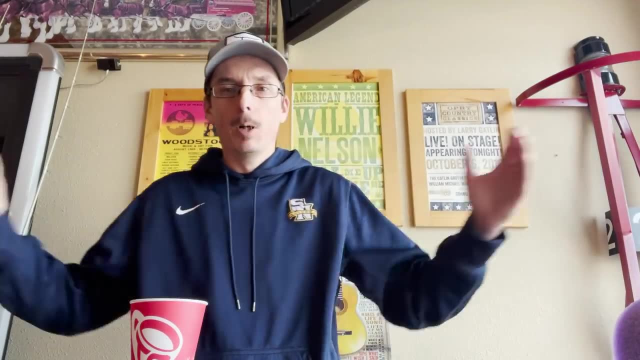 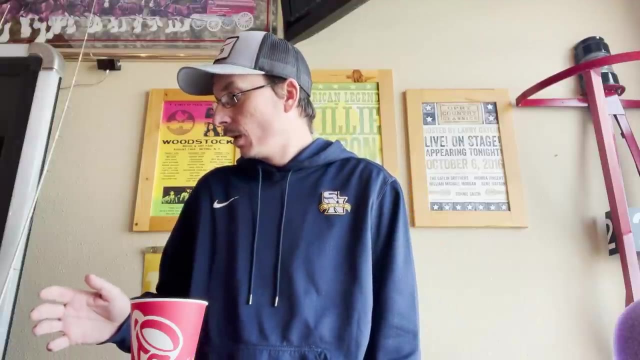 we got six planer board setup set up with quarter ounce inline sinkers as you can see here: quarter ounce inline sinkers, 15 pound mono lead about a rod length, so it's about eight foot. so you can easily lift your rod up and net the fish and then we'll have a ball bearing swivel on the business end. 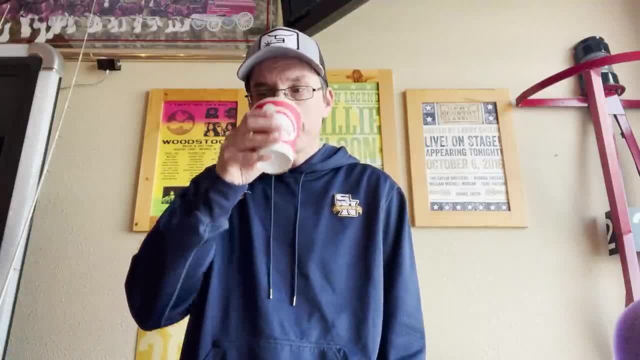 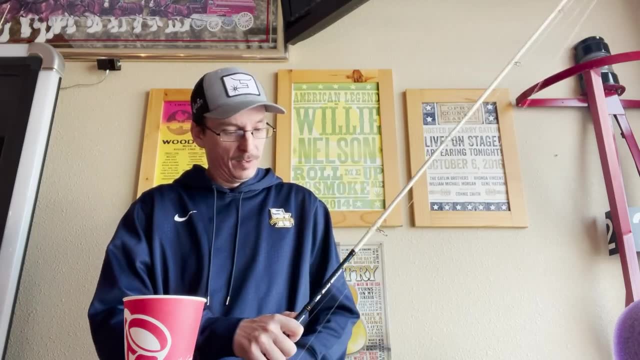 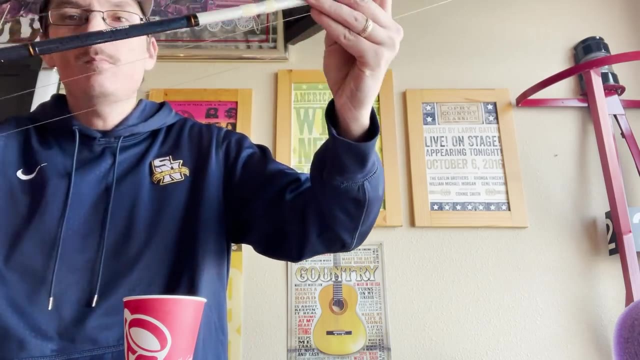 so that's, that's the planer board setups. now the diver setup, as I mentioned before, he uses the same rod, but in an eight six model, so it's a cold water. eight foot six. let's see if I can get this. it's hard. we got a window right there. I apologize. 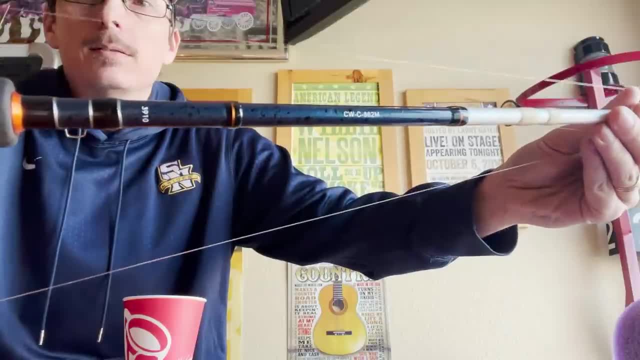 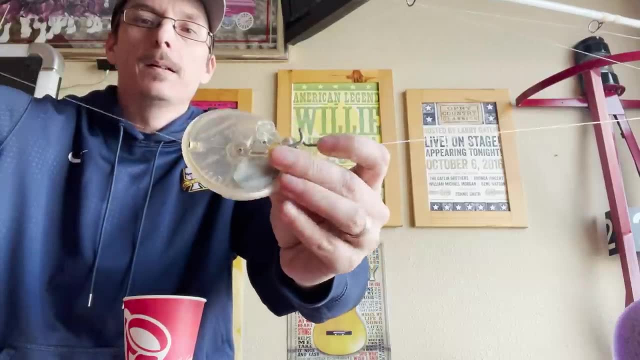 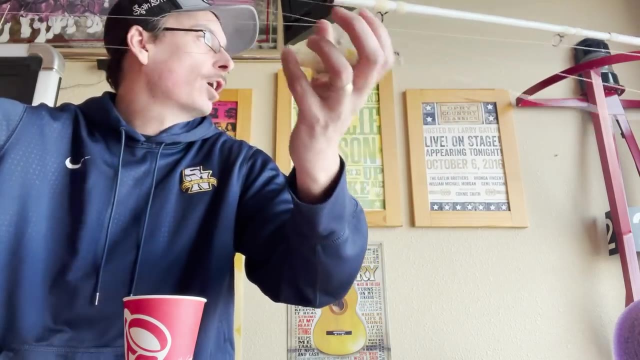 so it's a cold water. there you go, you can probably see eight foot six medium action rod again, and here what we're dealing with is we're dealing with a mini, which is a double zero slide diver. I call it the mini. the mini slide diver and slide divers are a. 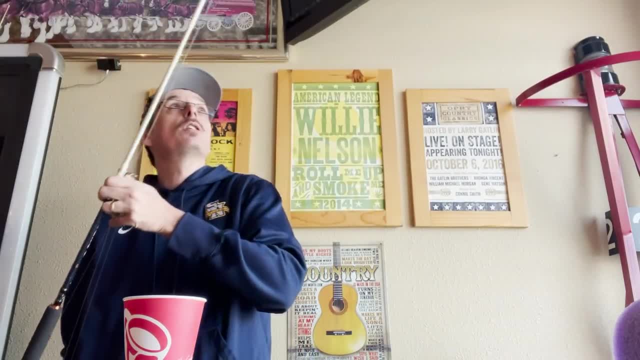 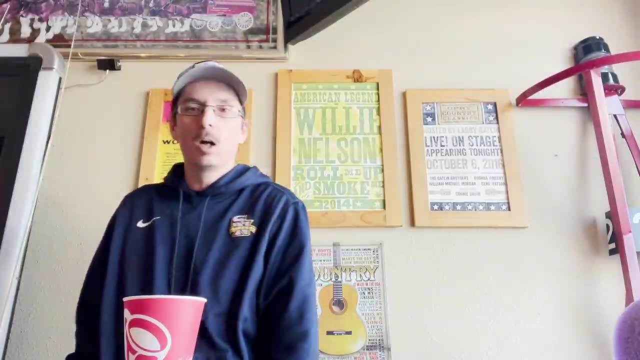 and slide divers are a. and slide divers are a critical aspect to spring brown trout fishing and i have a slide diver video on my youtube page. so i'm not going to go into a ton of deal about what a slide diver is or how it works, but there is a. 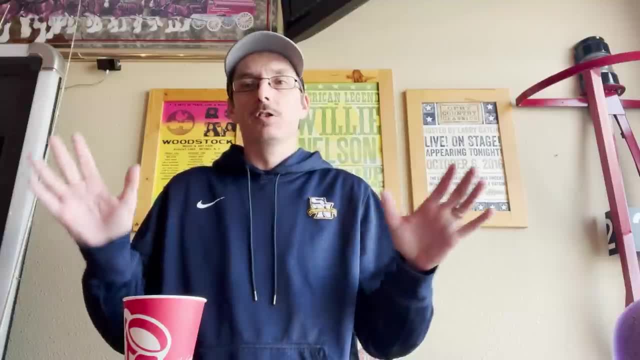 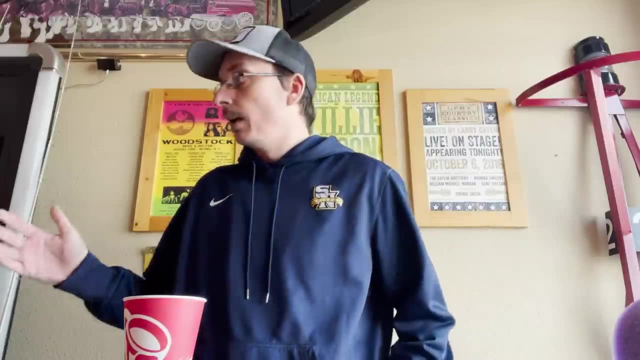 lot of days where that slide diver is going to be your hottest rod, especially if there's a little bit of boat action, you know, a little bit of waves, and or if you have a little bit of stained water or cloud cover. there's a lot of times where the slide divers might actually be even your hottest. 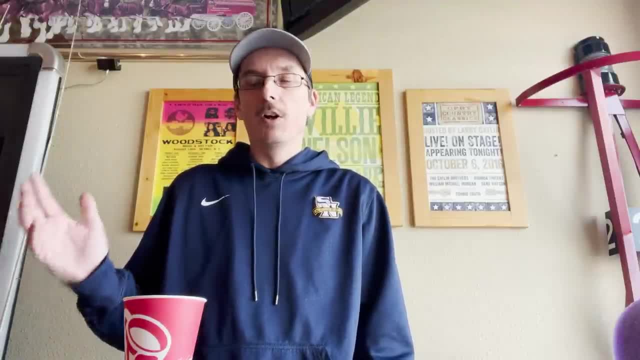 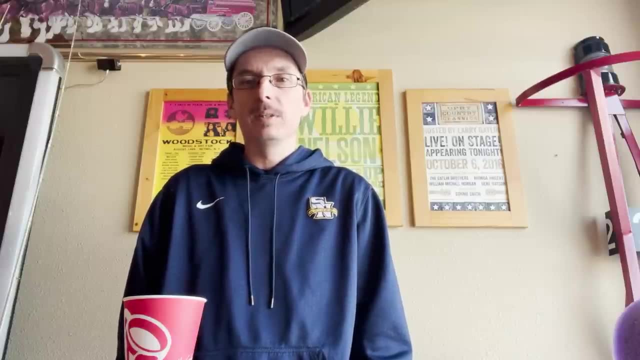 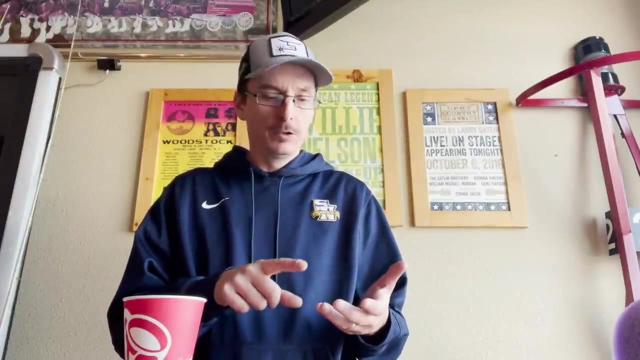 rods more than your boards. your boards will be very, very good all the time, but will be really good when the water is pretty clean and you and you're needing to be stealthy. so that brings us into tackle. i mentioned before that you know you can use junior thunder sticks, rapalas, bayrad crank. 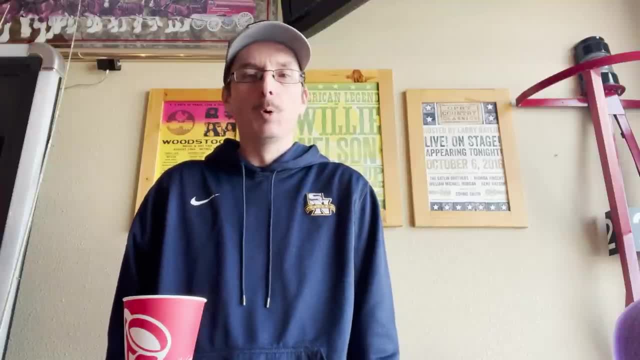 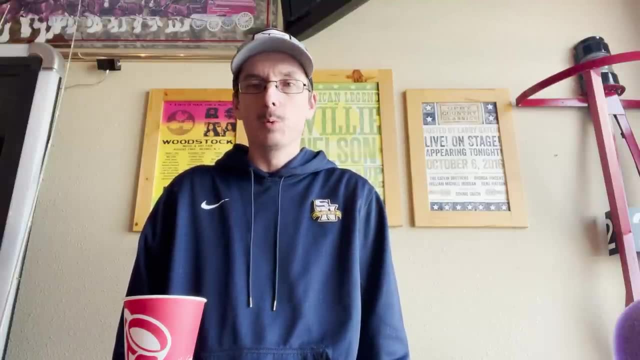 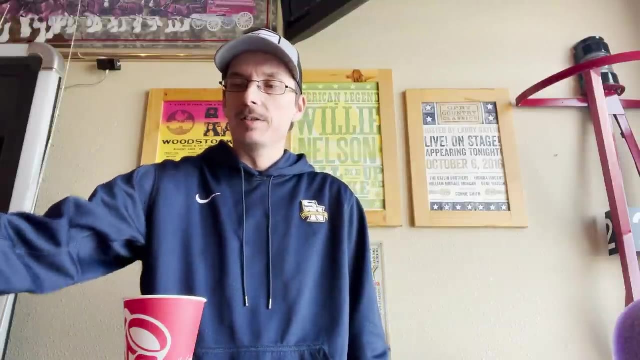 baits. all kinds of different stick baits or crank baits will work. flicker shads work great. all kinds of different crank baits will work and they have their days. but for me in particular, i prefer spoons. so when we came out with the salmon candy spoon series last year, a big part of that series was 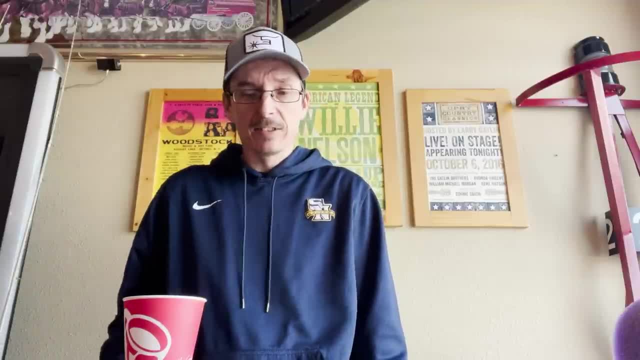 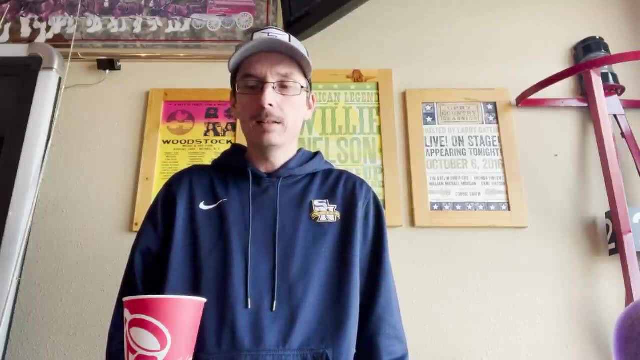 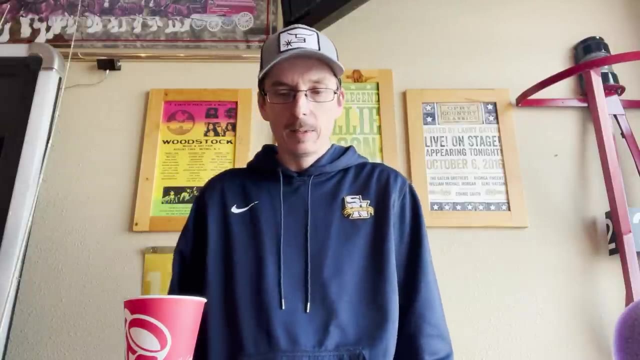 the mini spoon, the smallest one, and that spoon was designed with basically spring brown trout and spring cojos- but mostly spring brown trout- in mind and doubling up for a walleye spoon as well. so i'm going to go through some patterns here and kind of give you guys a little bit of a hand. 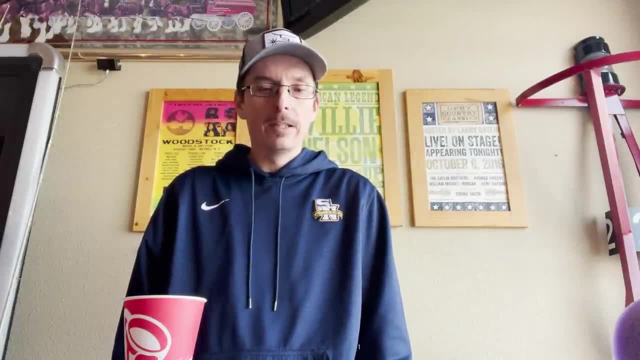 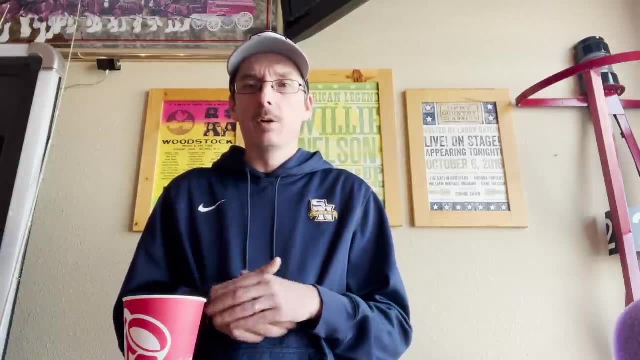 on what i would pick in different conditions. okay, so if we're going to go out today and when you're in that you know 8 to 15 foot of water. as you can imagine, the water is very clear nowadays on the great lakes. a lot of times you're dealing with situations where 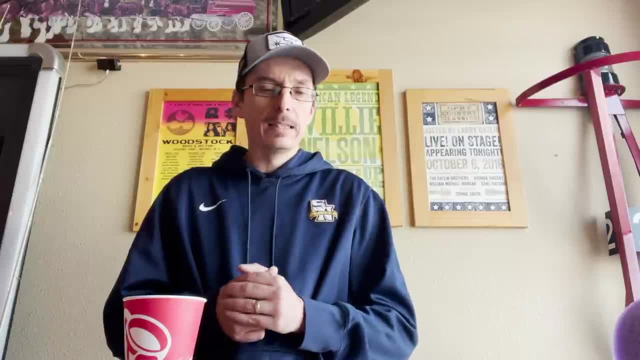 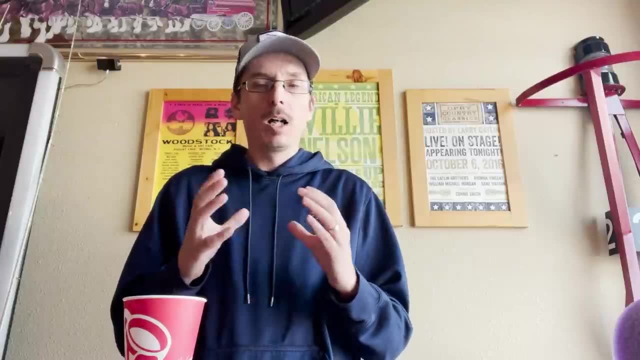 you may even be able to see the bottom, which is not ideal. you're generally not going to probably have a very successful fishing trip if that's the case, but we do deal with some of that when the water is clean or fairly clean. here are some of the patterns that i prefer. 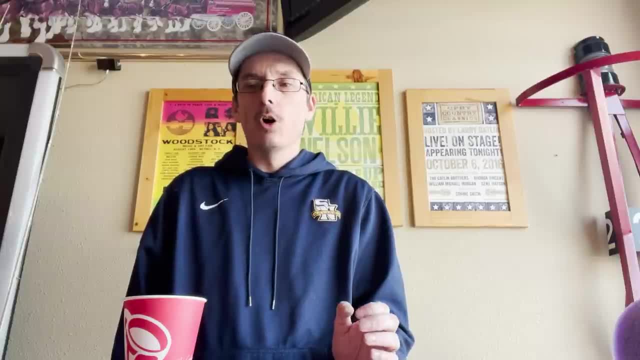 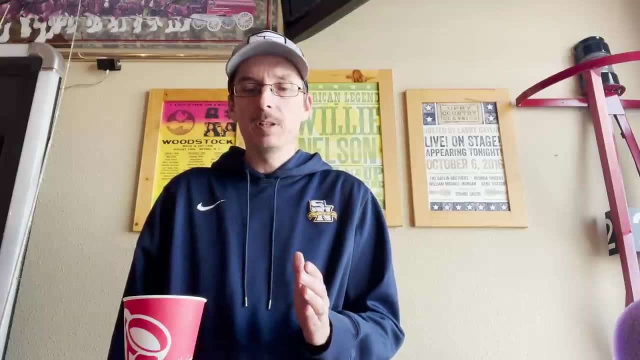 and actually let me rewind for a second. let me start off by saying i use almost exclusively gold and copper based spoons. now i may have some examples out here in silver that i grabbed, but i almost use almost zero silver mini spoons anymore for brown trout. i like them for other. 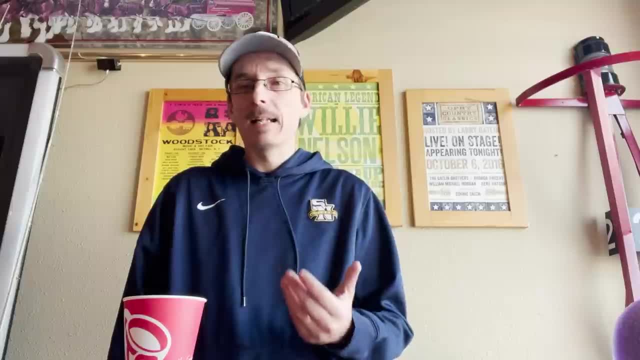 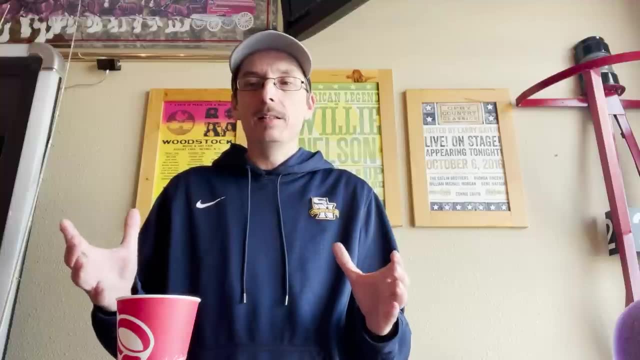 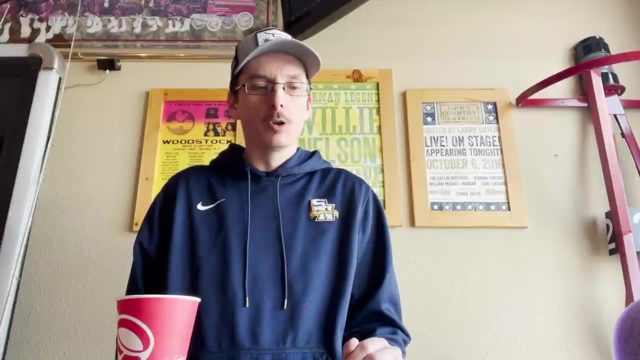 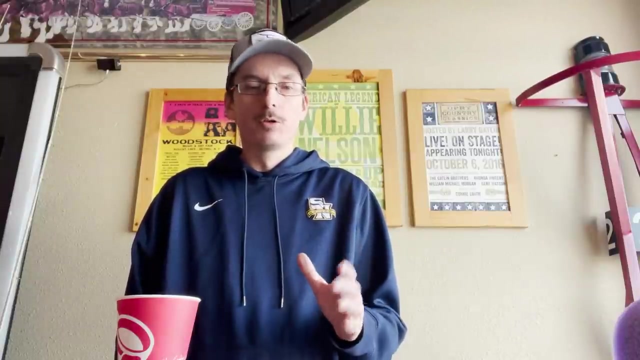 species, steelhead at times, cohos at times- and i'm not saying silver ones won't work. i'm just saying because of the round gobi being the forage base and it has a brownish, copperish look to it- or copper backed or blanked spoons tend to out produce the silver ones for the most part. so if 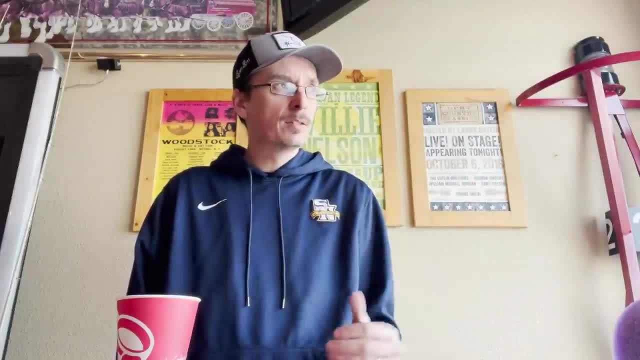 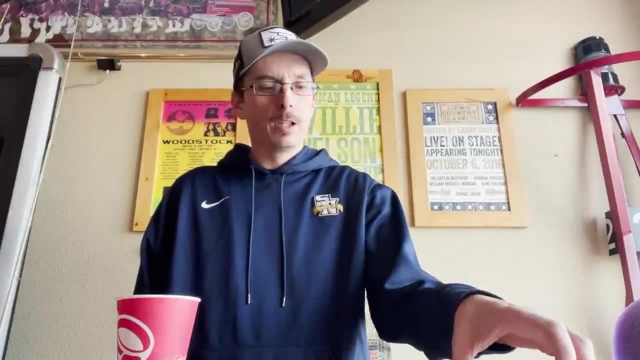 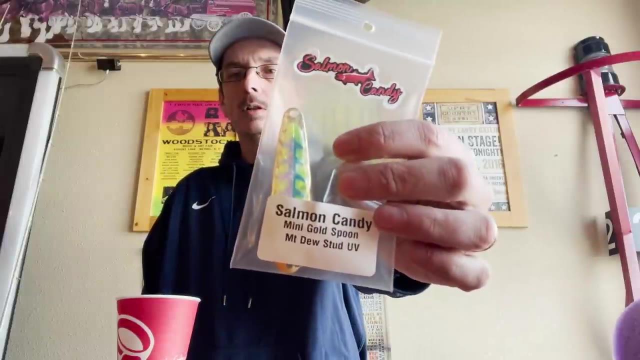 we're dealing with clear conditions today. uh, you know, we got bright, sunny skies. water's fairly clear. i can see two, three, four feet, for sure, down in the water column. these are some of the spoons i'm gonna pick. i'm gonna pick something like a blue mahi, you know, spoon um uh, mountain dew stud. 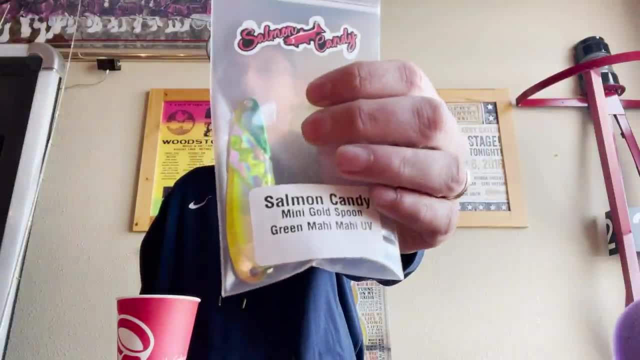 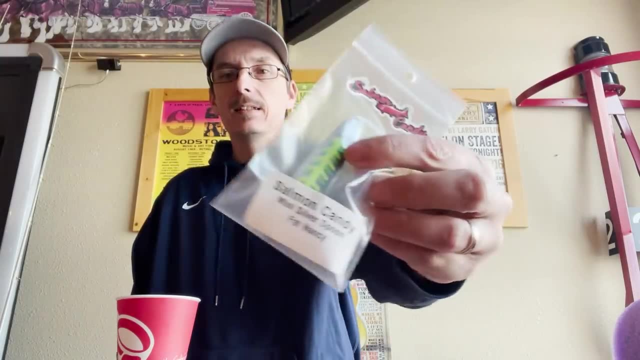 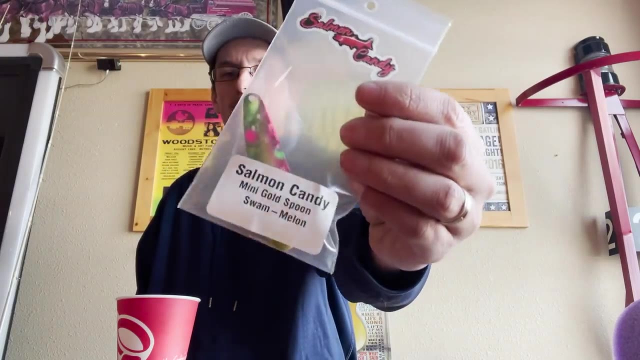 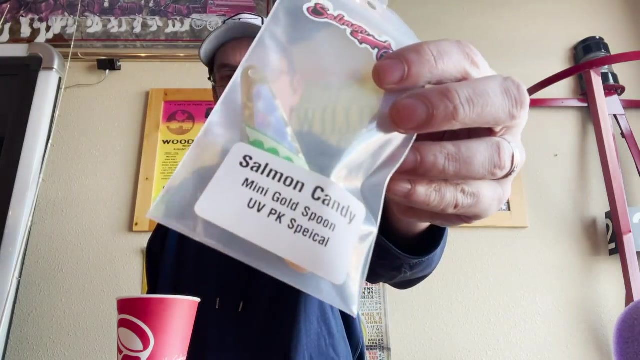 spoon, a green mahi spoon. you know an orange jeans fat nancy swamp melon. you know which is our version of a watermelon, which is a little bit different um than the average one, um pk special, which is a fantastic spoon. and then one of my favorites in clear water is the uv two-face. 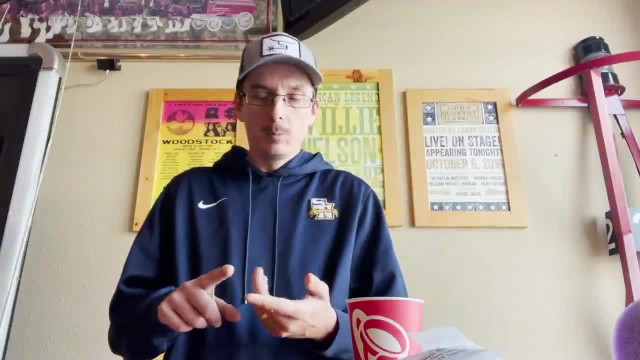 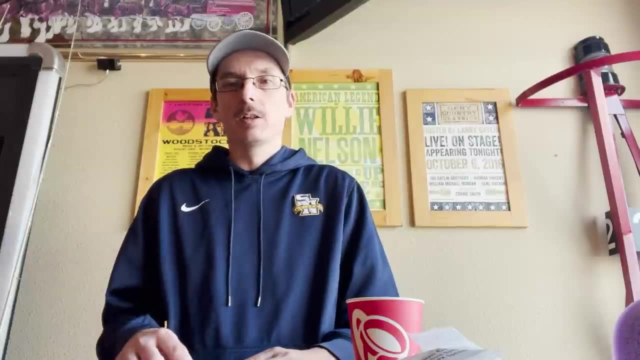 now in the spring, because it's springtime, we're dealing with weather, we're dealing with wind, runoff, all kinds of things like that, i would say. the water is stained more than it's clear, which is a good thing, because that's when the fishing is generally at its best. 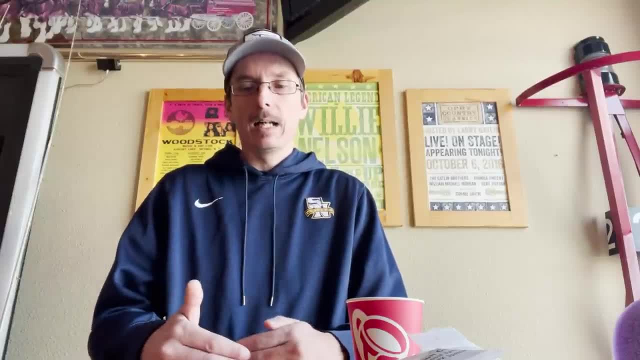 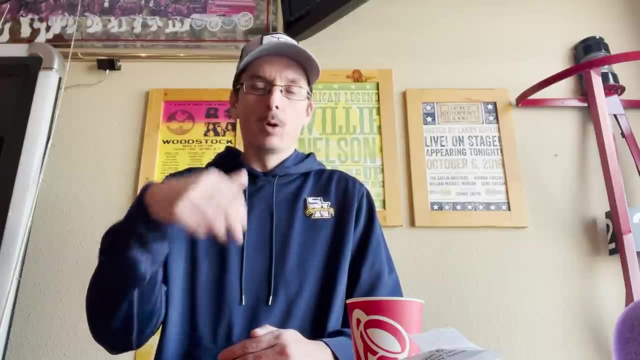 now there is a point where the water is too dirty and here's kind of the way i tell: if you have a smaller boat with an outboard motor, if you look down at your big, your big motor, your outboard motor, if you can see the prop on your outboard motor, then the watercolor is about perfect. 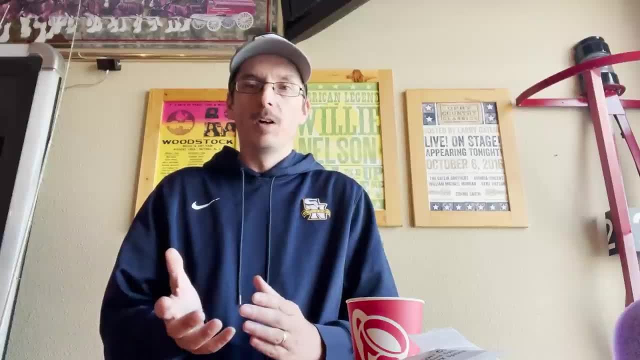 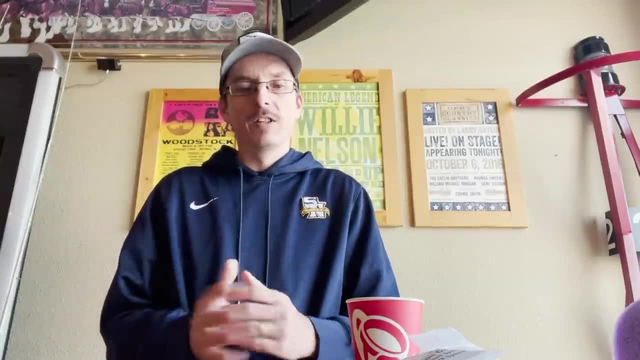 if you can basically just barely make out the prop, it's about perfect. if it's too dirty to see the prop in your outboard motor, it might be too dirty for you to have success catching fish. and, like i said before, if it's crystal clean to where you can see the bottom and read a newspaper. 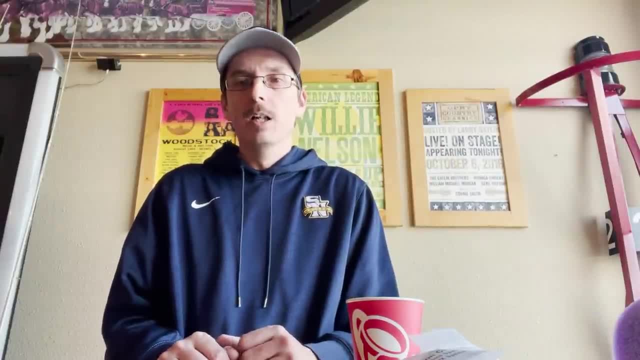 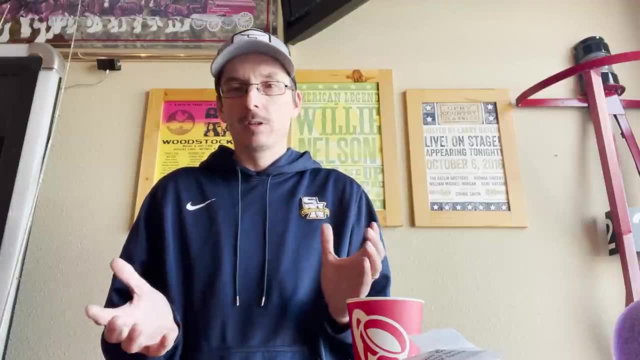 on the bottom and 15 foot, you're probably going to struggle a little bit. so ideally you want that middle range where you have some color to the water, but yet you you don't have crystal clean water, and that's why harbor areas at times might be some of your best fishing, because 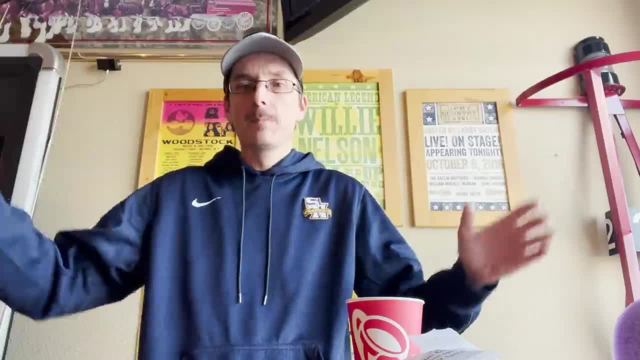 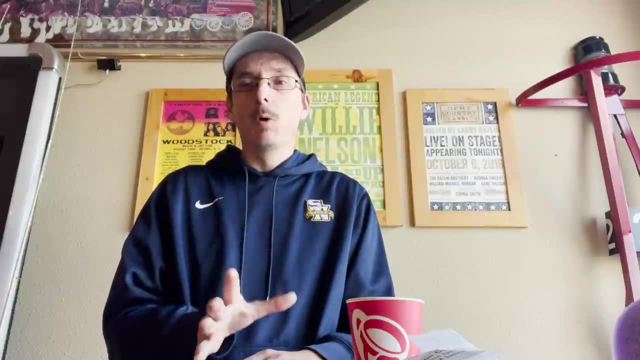 even when it's crystal clear. you know, in other areas you may have some dirty river water pumping out that you can fish to kind of fool the fish. so now, when i'm dealing with some stained water, here's some of my favorite colors, which is these end up being some of my all-time favorites. 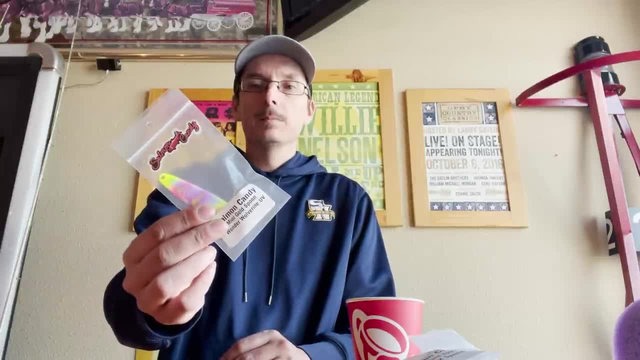 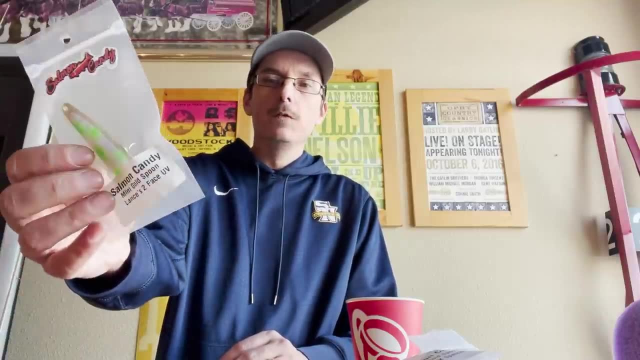 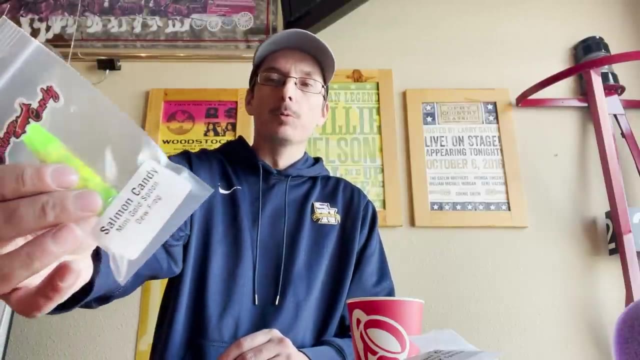 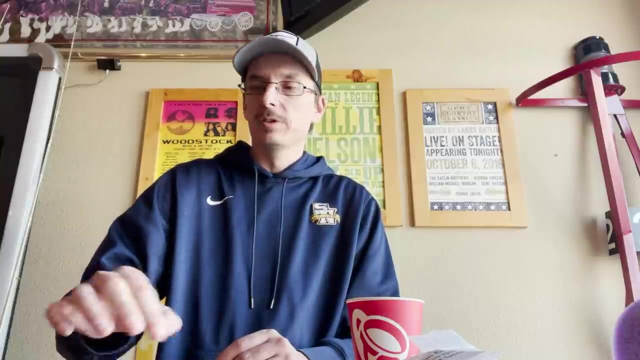 here for brown trout which are like wonder wolverine um orange crush lance's uv two-face, which is an awesome mini spoon that's double-sided, real gaudy kind of spoon. dew frog, which really produced last year for me in dirty water, produced for coho's down in wakigan, produced for browns every time i fished it. 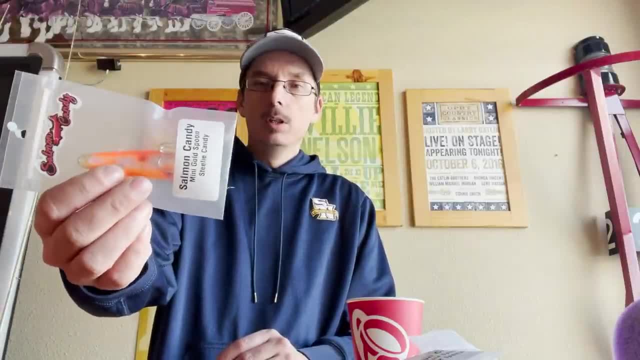 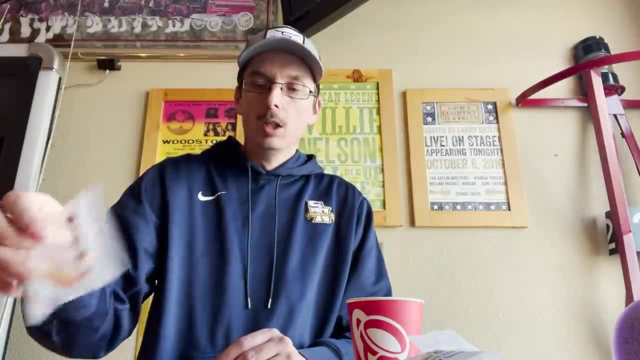 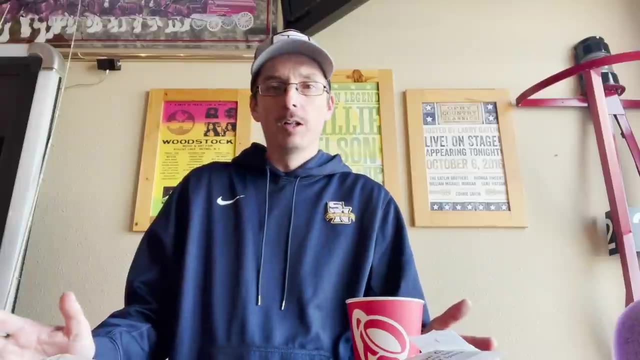 steely candy, bright orange gaudy spoon and then stud uv- that's another bright orange kind of real gaudy spoon. so those are some of the particular patterns i would select when i had a lot of color in the water, and then the ones that i showed you before is what i would go. 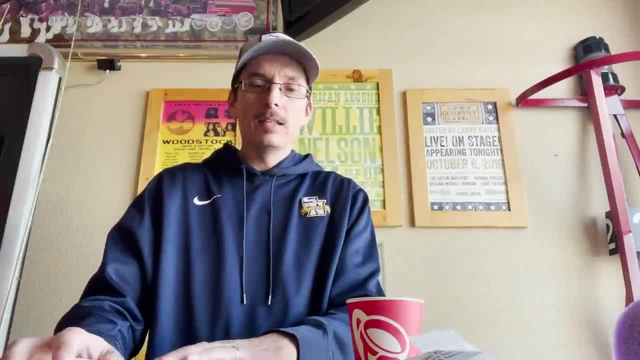 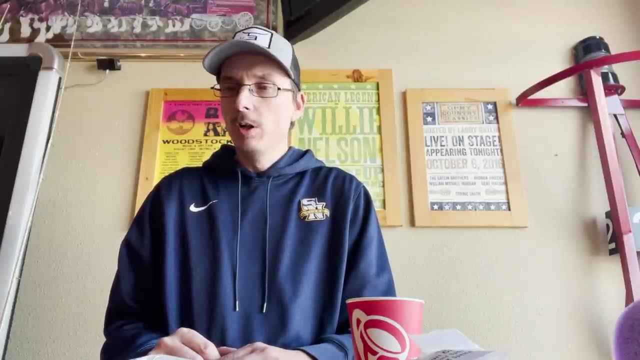 to when i did not have very much color in the water. now, let's say you get out there and you can barely make out your prop and you're like it's, it's dirty today. um doesn't seem too dirty that i probably can't catch fish. i'm maybe getting a couple of bites and i tried russell's dirty. 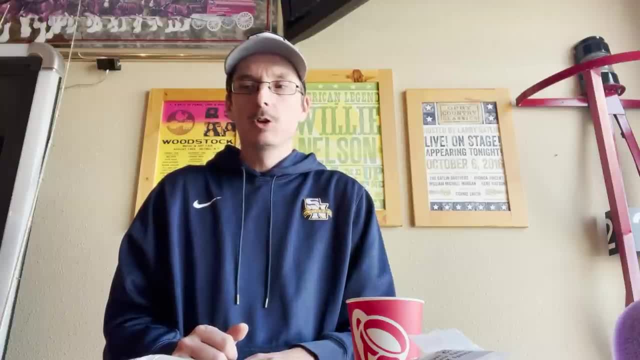 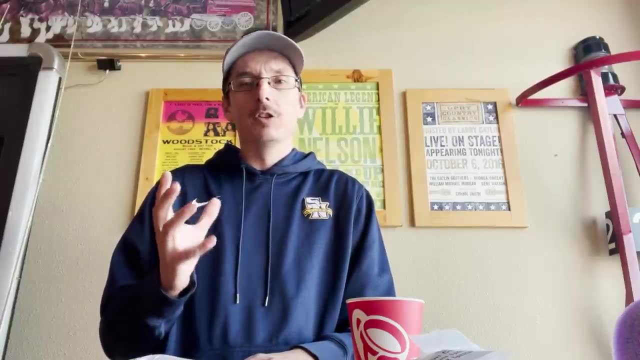 watercolors and i'm getting a couple of bites on them, but they haven't been crazy good. what else could i do? well, you could step up to a standard size spoon- and this is not something that i do very often, but if you're dealing with more dirty conditions, you can go to a little bit. 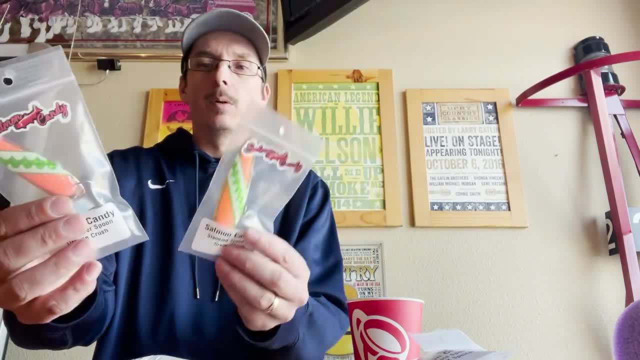 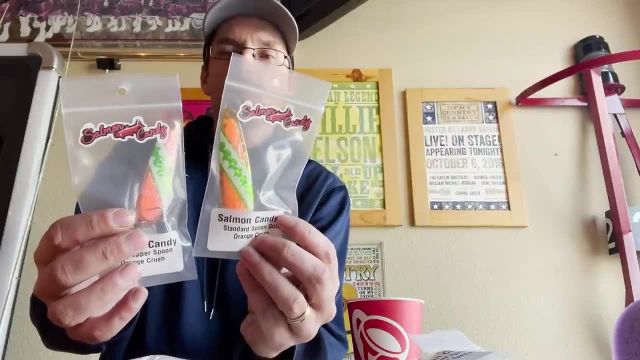 bigger profile. for example, i'll just show you. you know, here's an orange crush in the mini and an orange crush in the standard size. you know there's a perfect example. so you could bump up to that standard size orange crush spoon and that's going to help you probably get a little more profile, a little more. 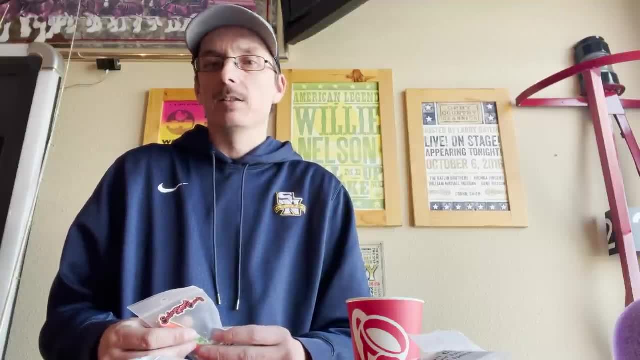 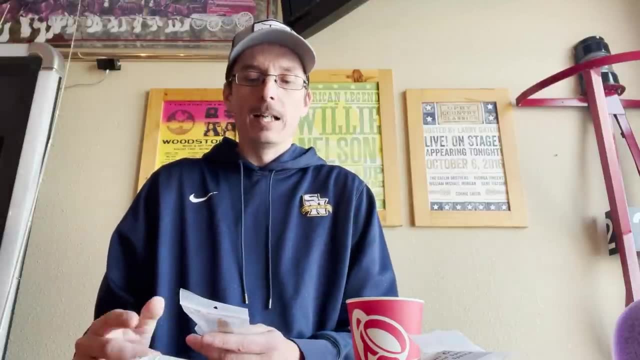 kick and turbulence in the water might attract a few more fish in that dirty water. i'm not a big fan of standard spoons when it comes to browns. don't bite them, especially the bigger browns, but i do think when the water is dirty it'll help, so you can go to. 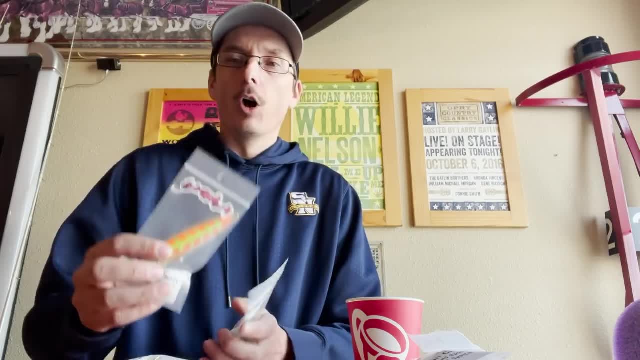 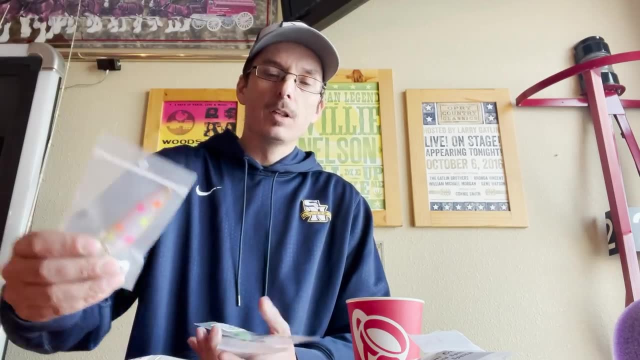 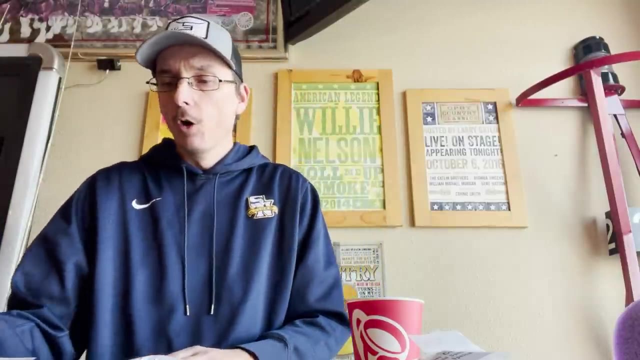 you know orange crush, uh, orange stud. you know all the same sort of colors, dew frog, you know all those types of colors, confusion which works in both sizes. um, you can go to a lot of those same colors, uh, in the standard size spoon and have success. so recapping now a little bit about brown. trout fishing in the spring generally starts happening as soon as we can put the boats in the water, which is usually early to mid-march, and then ends as soon as the bait fish flood the shore line, and that can be anywhere between mid-april all the way to the beginning of may we're going. 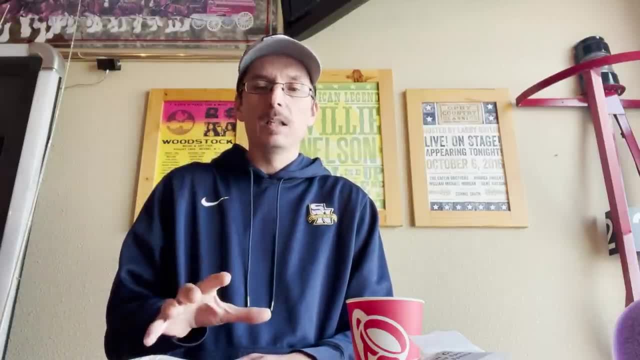 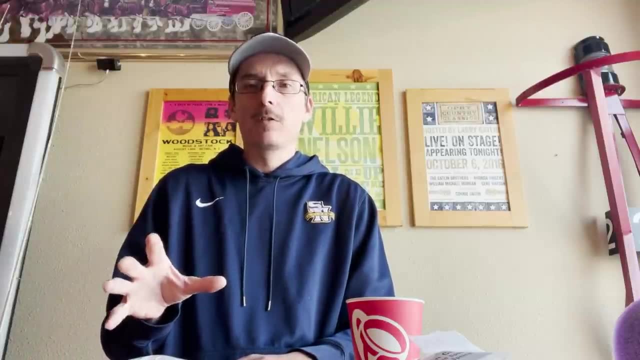 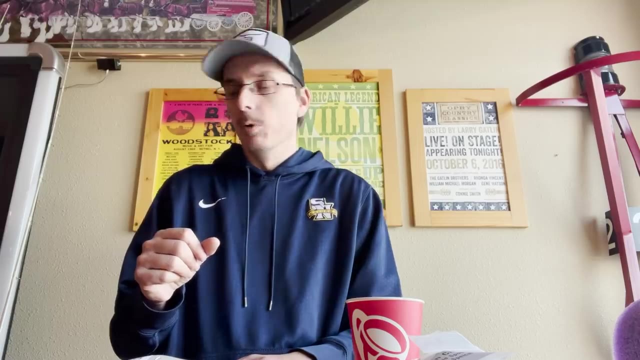 to generally use lightweight spoons like salmon candy's mini spoon, primarily gold and copper color. we're going to use rods that have real light action, preferably that bend a lot on these cold water. the browns are usually fairly aggressive, they got soft mouths and we're going to use inline 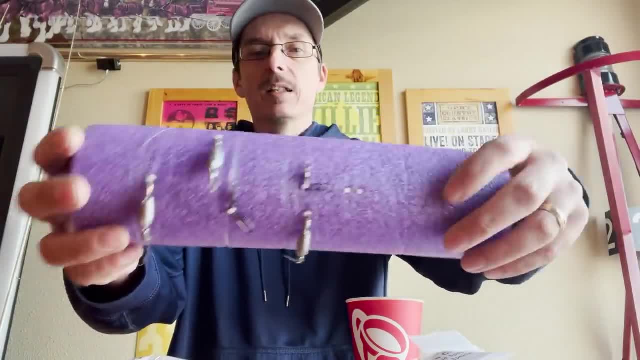 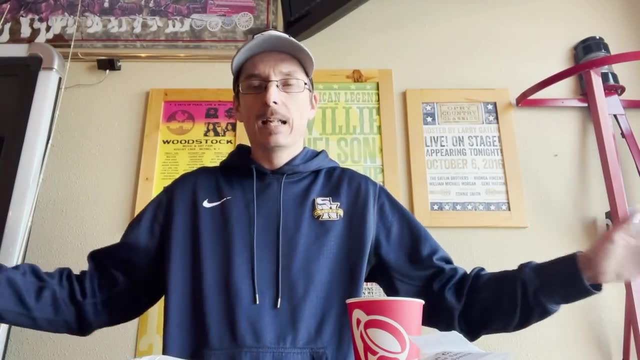 sinkers like quarter ouncers, um, to get us to get our spoons down in the water column, but not too fast. and then we're also going to use something like the mini slide diver as a diver type setup. a lot of guys are thinking themselves: well, what speed? well, you're dealing with extremely cold. 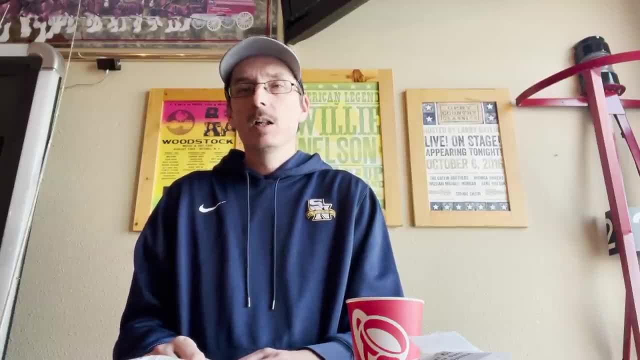 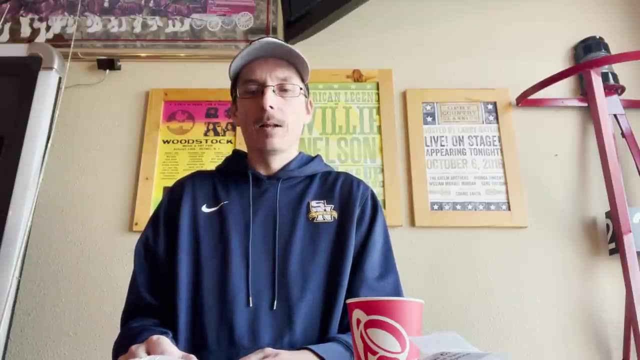 water. when you start fishing in march it might be in the upper 30s, low 40s and hopefully by the time we get you know into april, maybe it's approaching the upper 40s. so we're talking a lot of 1, 7 up to about 2.2 miles an hour, but in particularly i really like that 1, 7, 1, 8, 1, 9 range. now last year i poured brown trout fishing, i believe in april and that particular day they wanted it a touch faster. we tried that. one, seven, one, eight, caught a couple of fish, bumped the speed up to two. one, two, two. 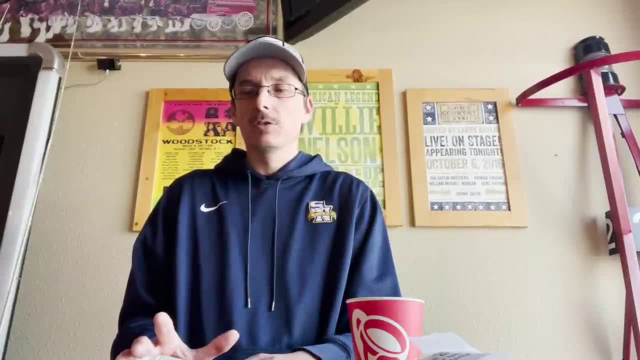 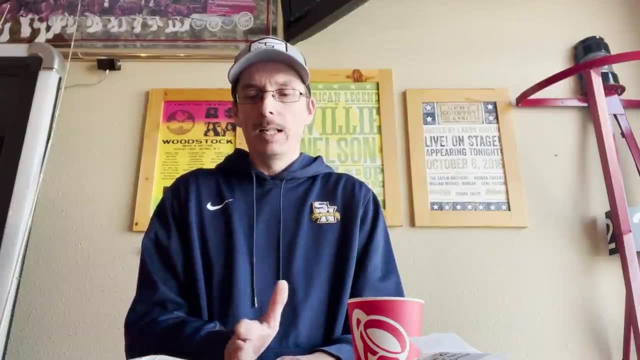 and we started cracking them. so, like anything out on the great lakes, you gotta, you know, gotta- treat each day a little differently, um, and see what they want that particular day. but i would say the range is about one, eight or, excuse me, one, seven to about two, two. that's kind of the speed. 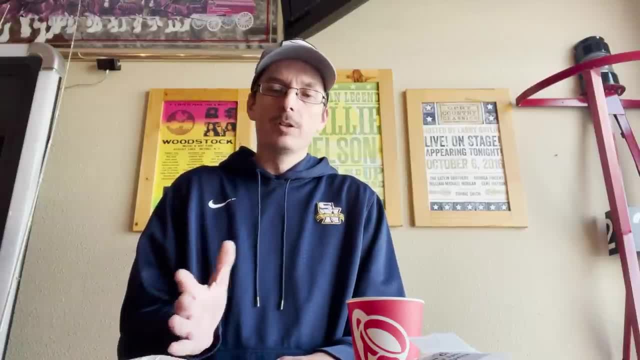 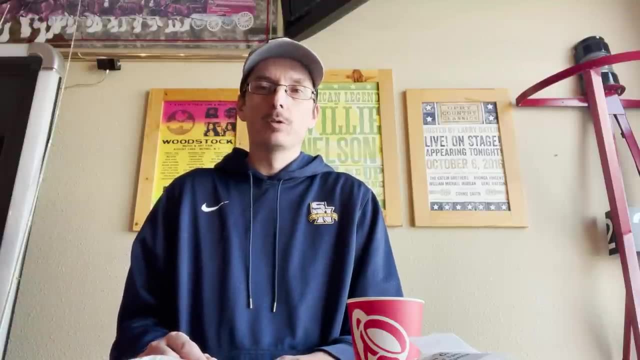 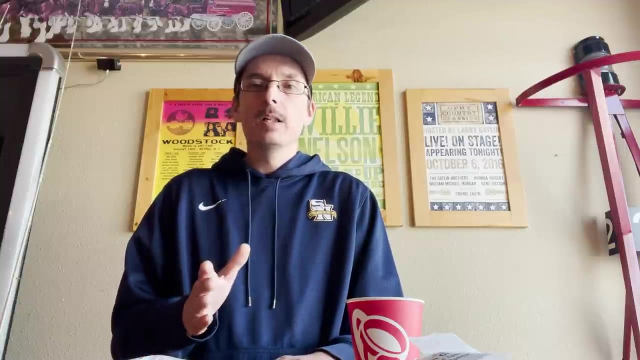 range you're going to use when fish and spring browns lean towards the slower side earlier, when up the speed a little bit towards, you know, the end of the brown trout. spring brown trout season, um, as we get closer to, uh, to early summer. so that's what we got for you today. spring brown trout tips. 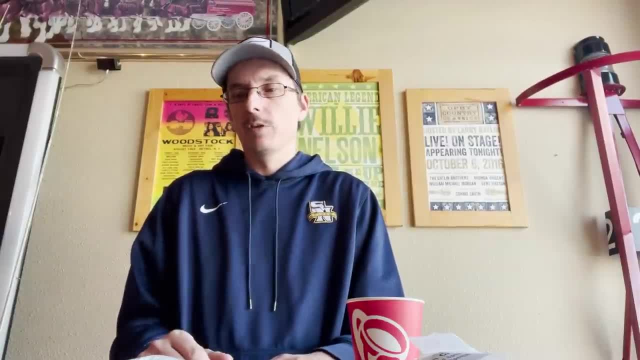 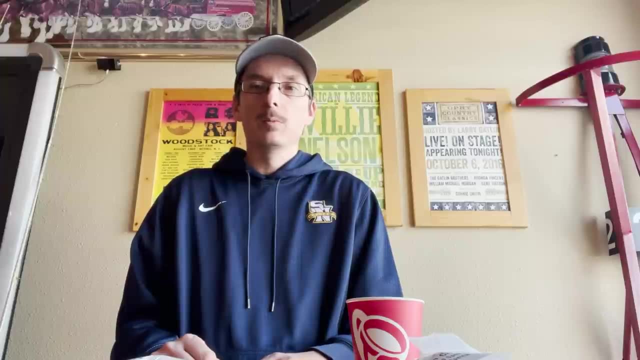 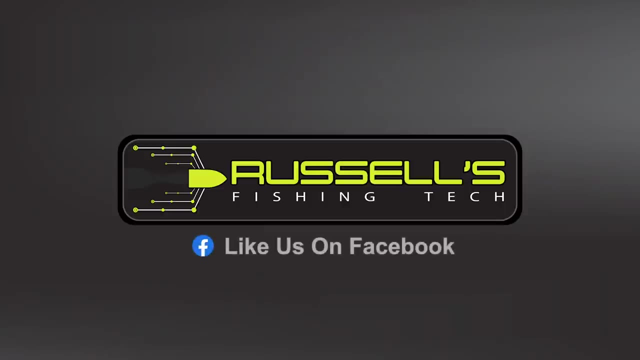 tactics and tackle. hope you enjoyed this video. remember, if you're looking for any of this gear, you can find us at wwwsalmoncandyfishingcom. check out my new uh website, which is wwwrussellsfishingtechnet. hope you enjoy this video and i'll see you in the next one.